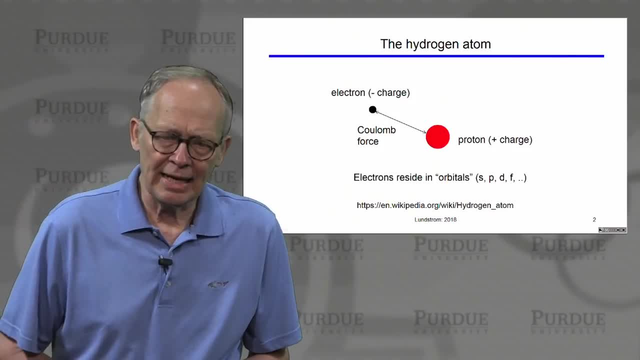 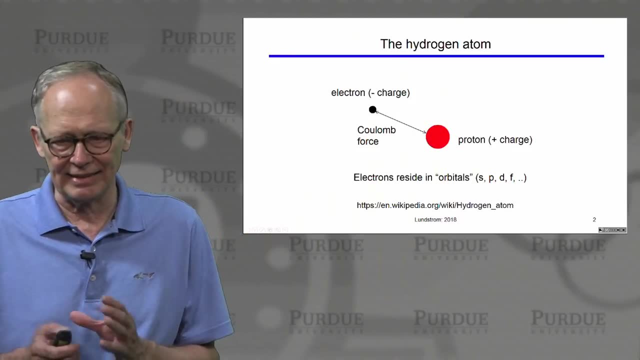 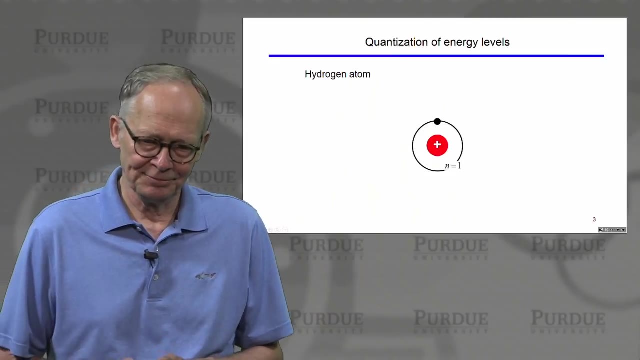 charges attract each other And you'll recall that the electrons reside in states And we label these states or these orbitals, sp, d and f you may recall. Now, another label for the states is the principal quantum number: n. n equals 1 is the lowest energy state, n equals 2 is a higher energy And the energy 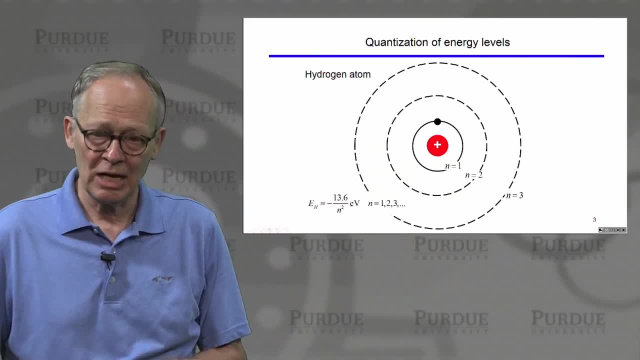 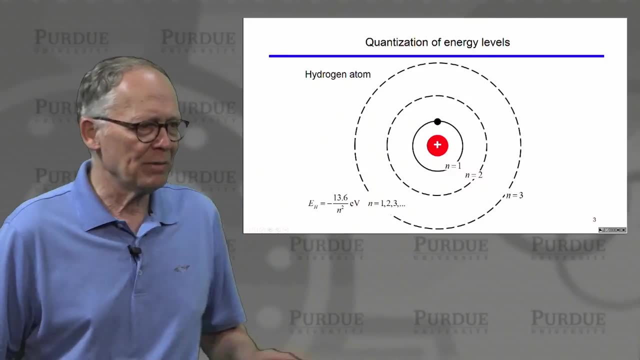 just increases as the principal quantum number increases. Associated with each of these principal quantum numbers is a set of orbitals, the sp, d and f. And you may remember this formula: The energy is minus 13.6 electron volts divided by the 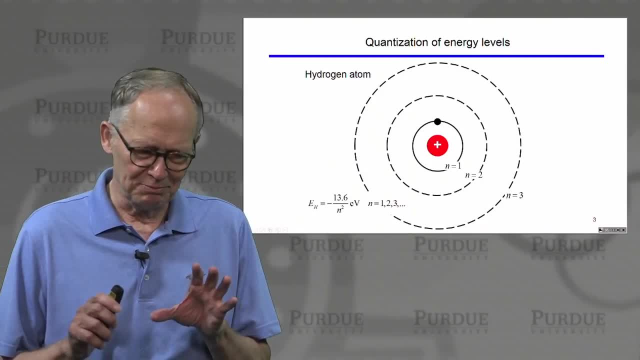 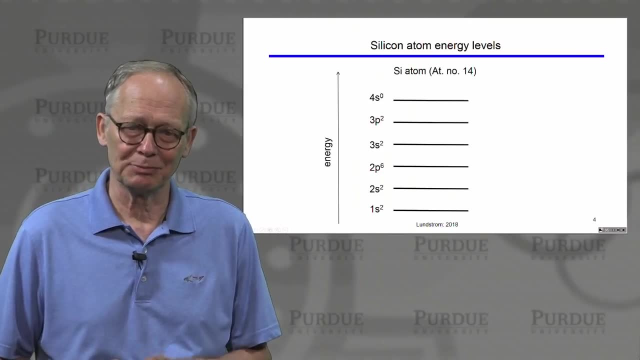 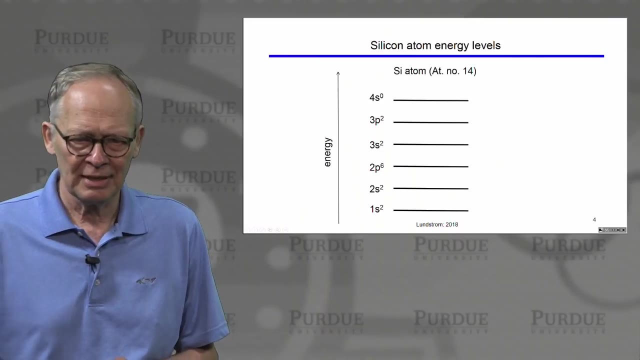 principal quantum number squared. So this is some basic fundamentals that we learned about hydrogen atoms. Well, silicon is the most common semiconductor. It's much more complicated than a hydrogen atom. It has 14 electrons and 14 positive charges in the nucleus. 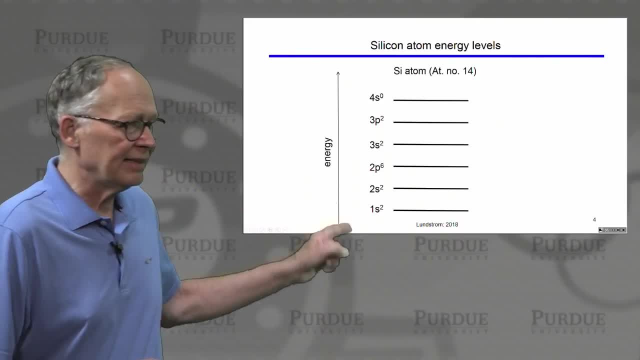 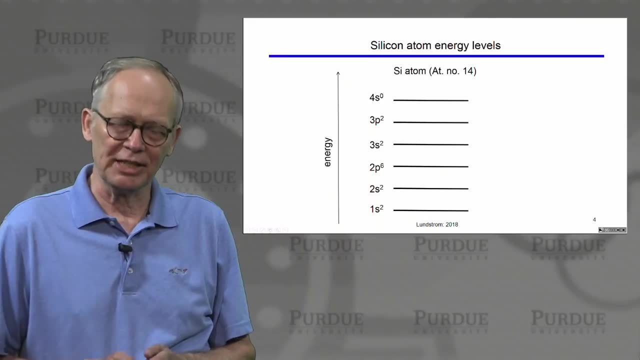 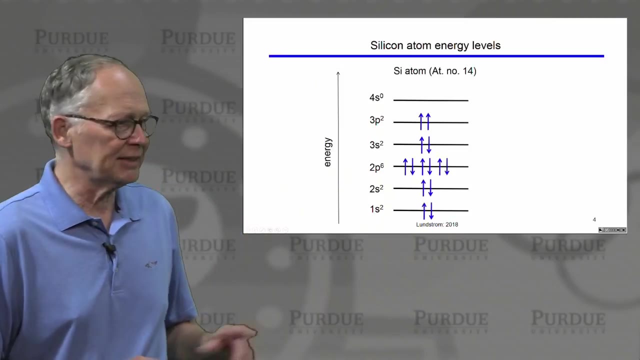 So if we ask where those electrons reside, they reside in a set of states labeled by 1,, 2,, 3, and 4, the principal quantum numbers, And associated with each of those principal quantum numbers is a set of orbitals. So we need to fill up the 14 electrons into those states. We 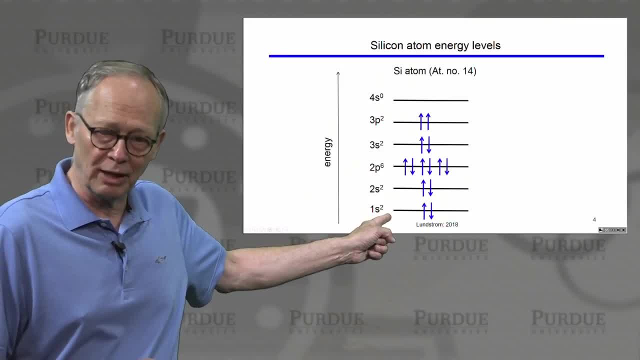 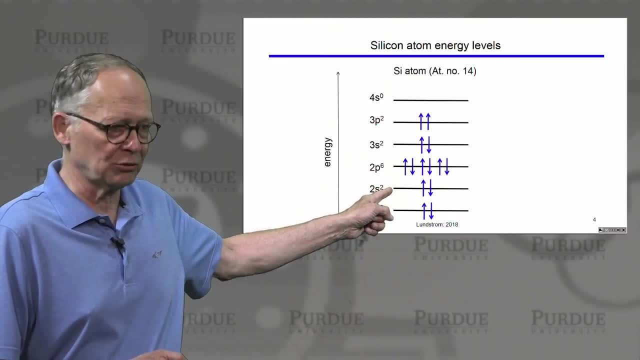 start at the lowest energy. We can put two electrons, One would spin up, One would spin down, in the s orbital for n equals 1.. We can put two more in the n equals 2 s orbital. You'll recall that the p orbital. there are three of them, associated with the x, y and 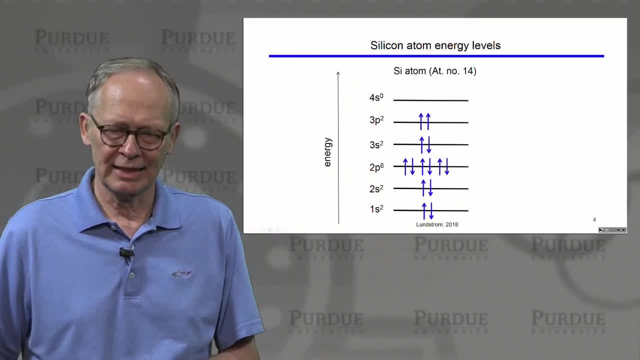 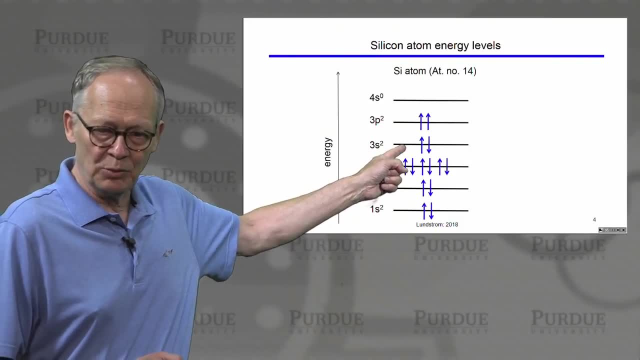 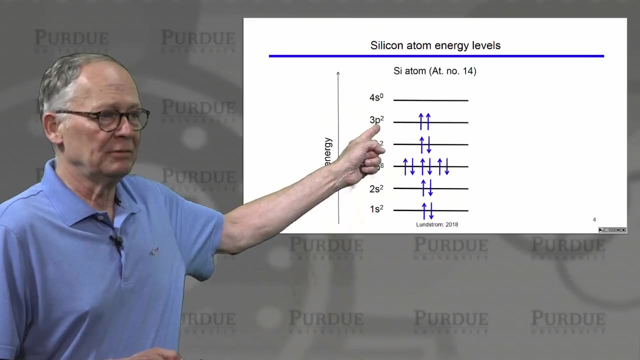 z directions. Each one of those can hold two electrons, So six electrons can be held in the p orbitals. So we can put six electrons in the 2p states. We can then continue to the n equals 3 states and put two electrons in the s orbital, And then we have six more states available in. 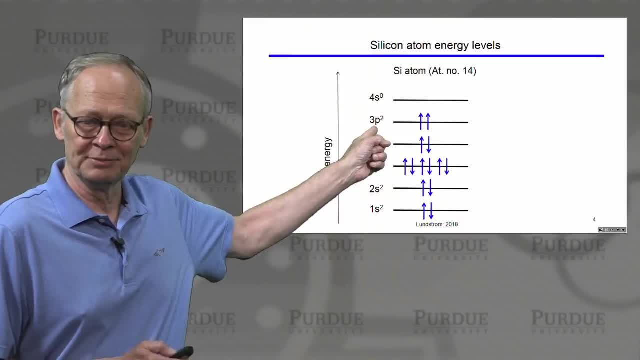 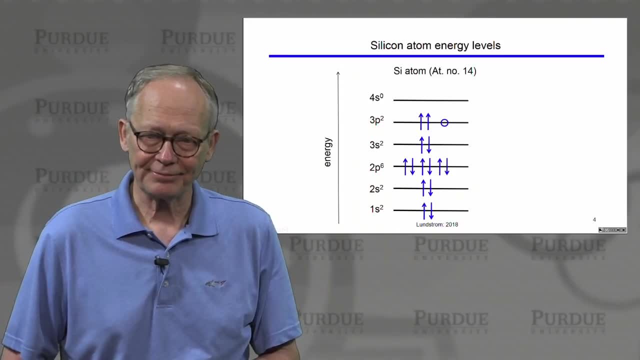 the n equals 3 level, But we only have two more electrons left, So we can put the two electrons in the 3p orbital and we have four states that are empty there. Now you'll recall that in the early 20th century, the way people sorted out this understanding, 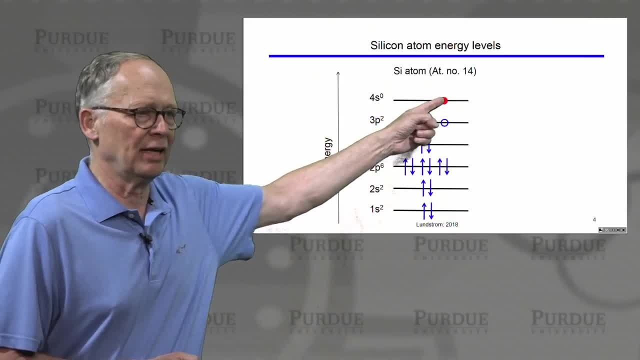 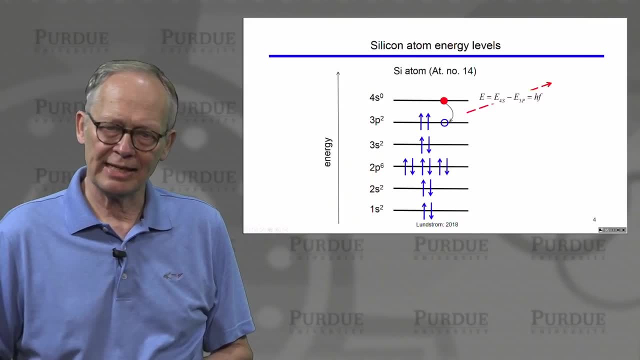 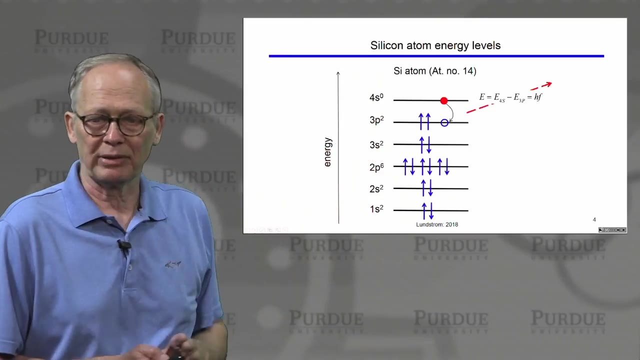 of atoms was by thinking of exciting an electron and putting it into one of the higher orbitals, letting it drop down and release energy. That energy comes off in the form of light. The frequency of the light is given by the energy difference is equal to Planck's constant H times. 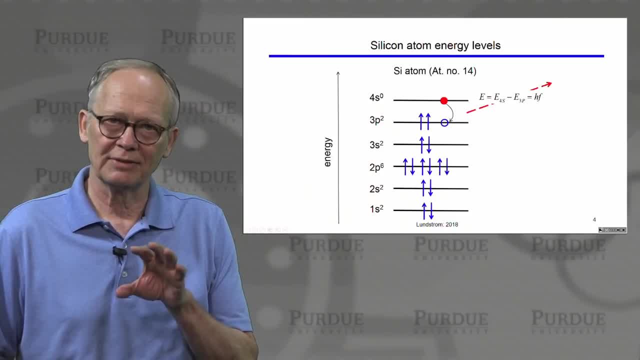 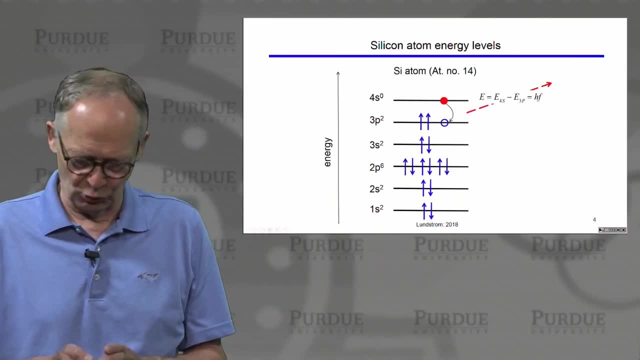 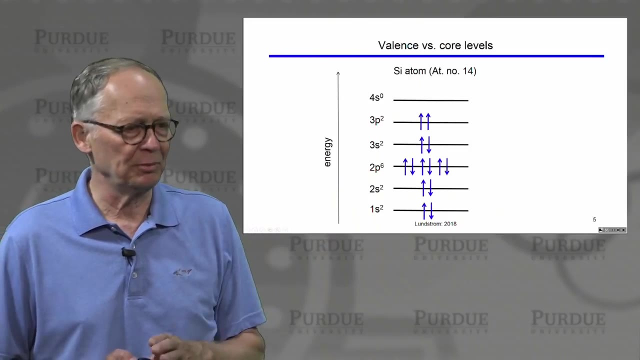 the frequency And understanding these discrete colors of the light that were emitted from the atoms is what led to the development of quantum mechanics and the understanding of these orbitals and energy levels. Now, this is a relatively complicated situation and we're not going to be. 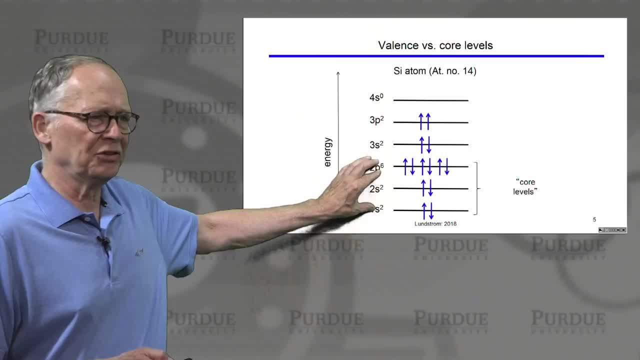 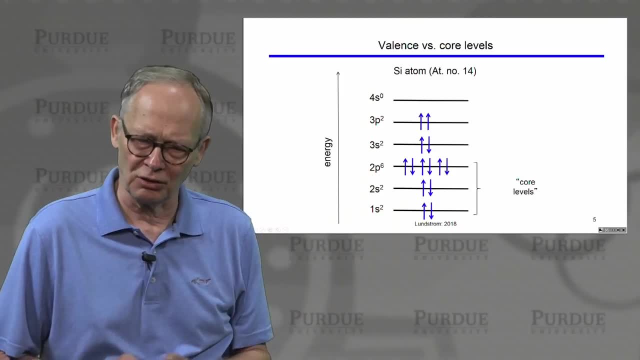 interested in most of it The electrons that are in the lowest energy states. these are bound very tightly to the core. They don't interact with the outside world much at all and they're not going to be relevant for us in this course. The electrons that we're interested in are in the highest energy. 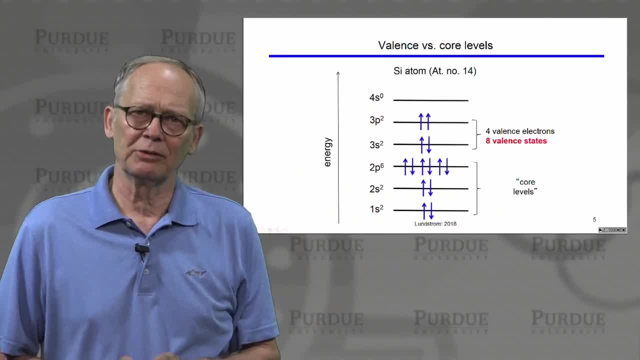 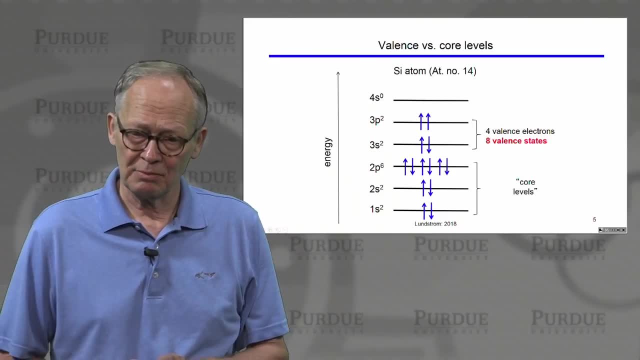 state. the n equals three state. These are the electrons that are responsible for chemistry and the chemical balance. These are the electrons that are responsible for the energy balance bonds. We call these the valence states. There are four of them in silicon, but you'll recall. 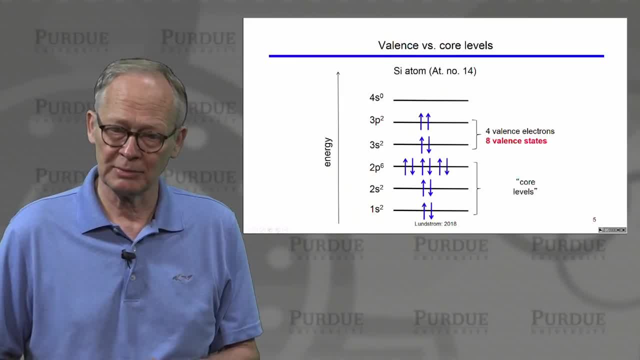 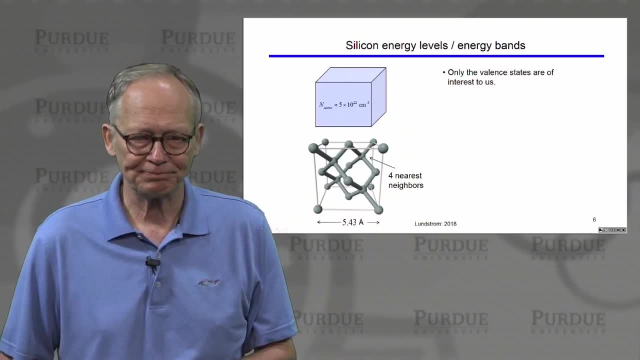 that there are also four empty states in the 3p orbitals. So we have four valence electrons, but we have eight valence states. Those are the ones that we're going to be focused on. So let's think about. what we're trying to understand is not an isolated silicon atom. 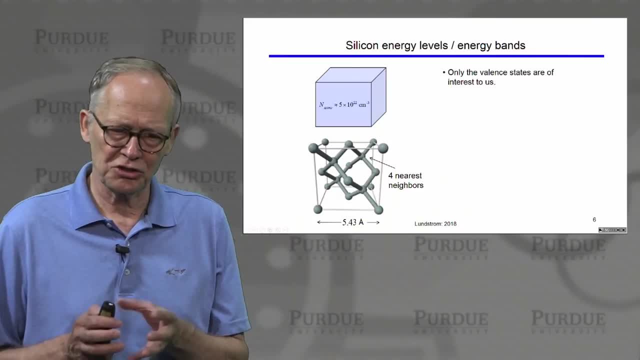 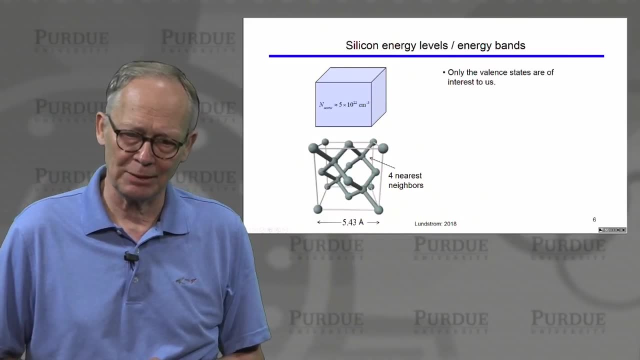 but a chunk of silicon crystal where there are a large number of atoms per cubic centimeter. So in a silicon crystal there are about 5 times 10 to the 22nd atoms per cubic centimeter And they're arranged in a crystal lattice that has a little bit of a complicated structure. 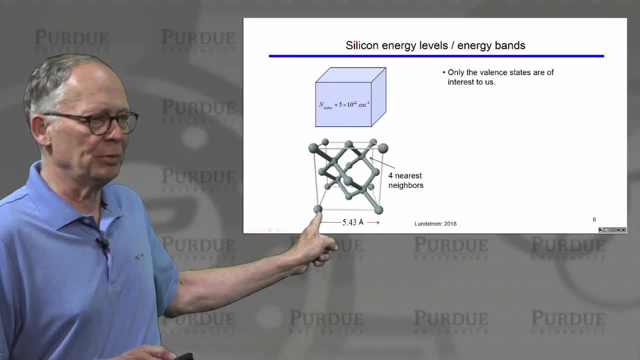 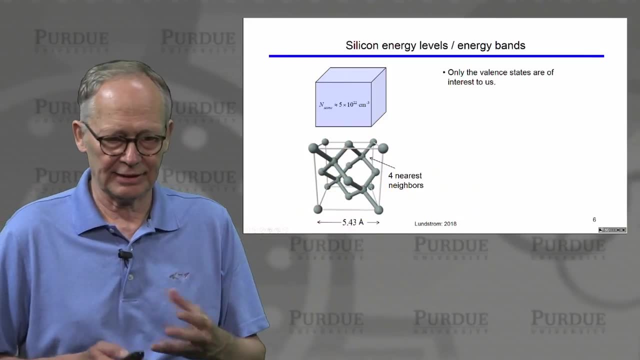 You can see it here. They're arranged in a cubic structure. There's a silicon atom at the corner of every cube, There's one at the face of each, at the six faces of those cubes, And then there are four more inside. If you look closely you can see that each silicon 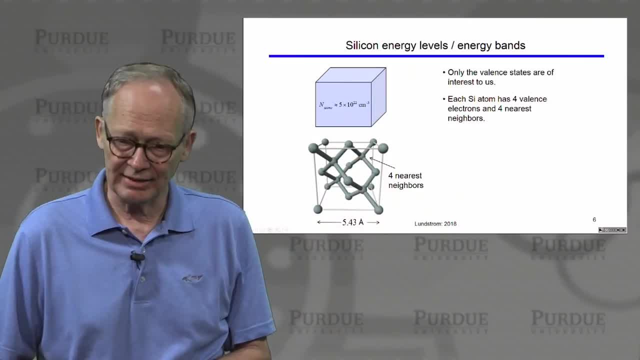 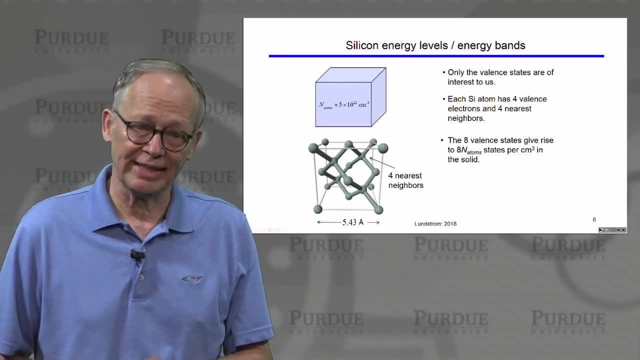 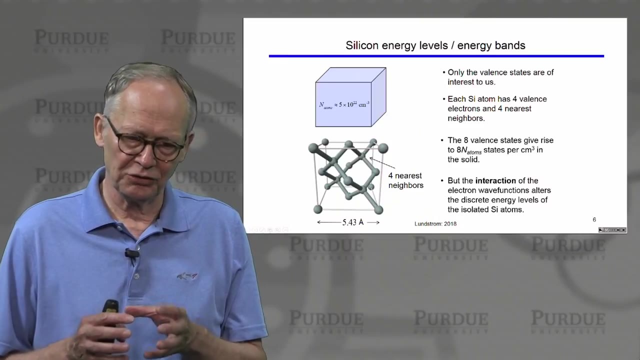 atom is surrounded by four nearest neighbors. Okay, And that's important. The eight valence states give rise to eight times the number of atom states in the crystal, but only half of them are filled. But something very important happens When the electrons are, or when the silicon atoms are put in a lattice a short distance. 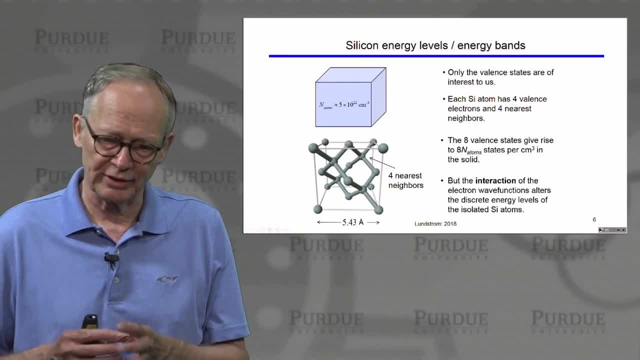 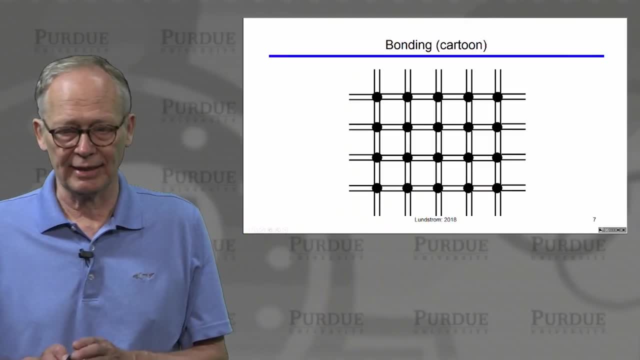 away from each other, the chemical bonds form and the orbitals interact and the discrete energy levels of the isolated silicon atoms change. In fact we no longer have discrete energy levels. But before we talk about that, let me just give you a much simpler picture of that silicon. 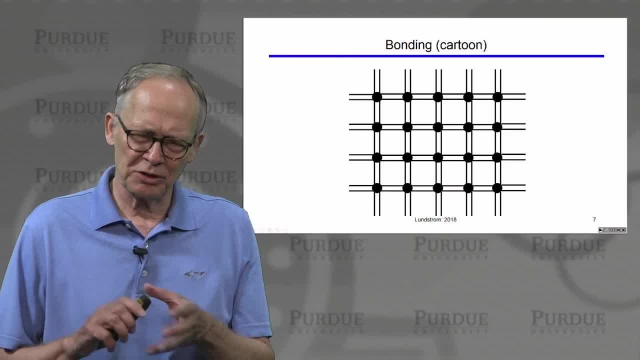 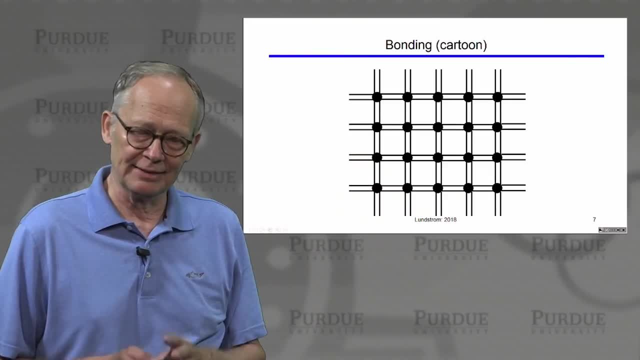 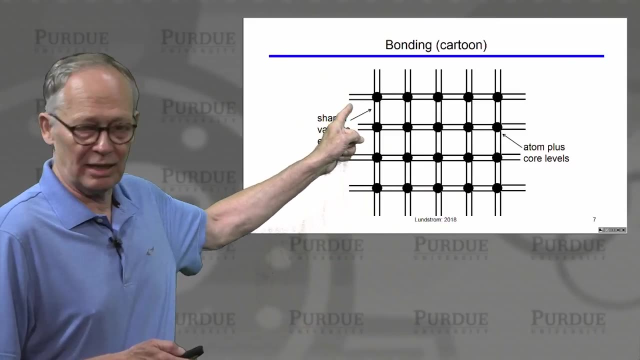 lattice that we'll use frequently in this course. Rather than drawing the complicated three-dimensional structure, we'll draw this little cartoon. The important point about the silicon or other common semiconductor lattices is that each atom represented by the black dots here, each atom- is surrounded by four nearest neighbors. 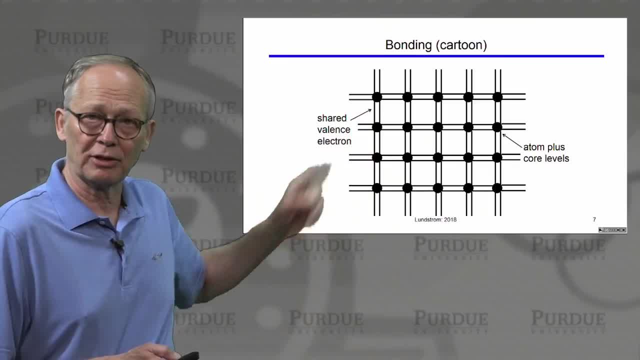 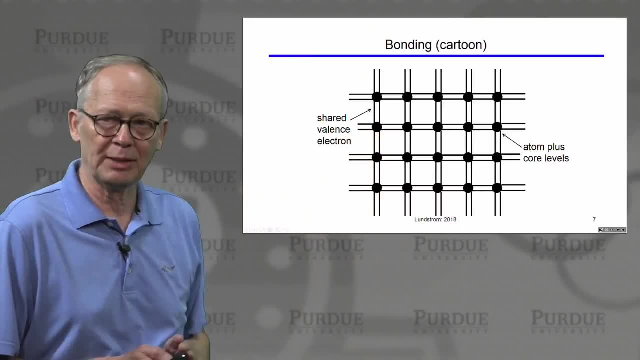 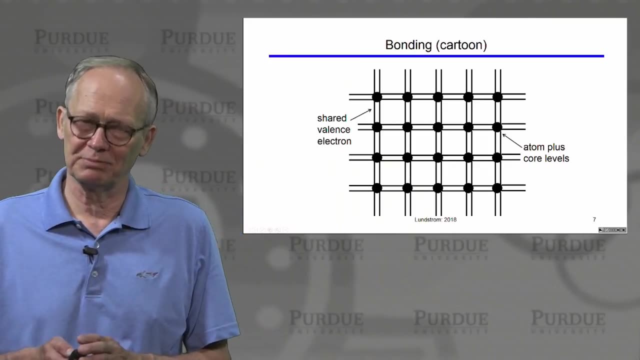 The lines here represent the valence electrons. There are four with each atom And if we share those valence electrons between its four nearest neighbors, then we effectively have the eight states that are available filled. That's the basis of a covalent chemical bond. 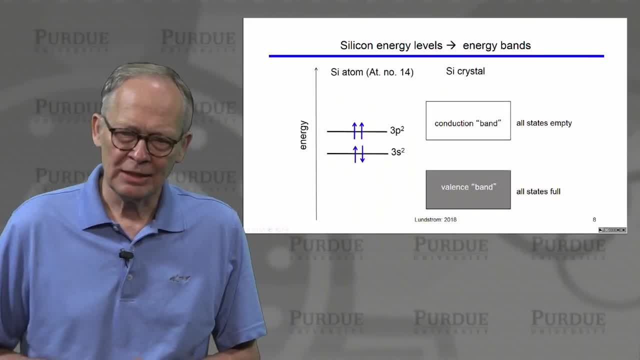 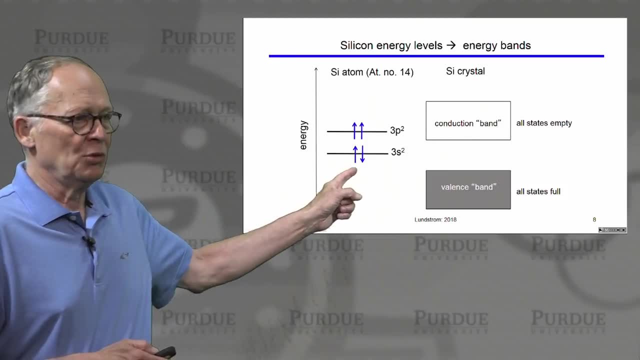 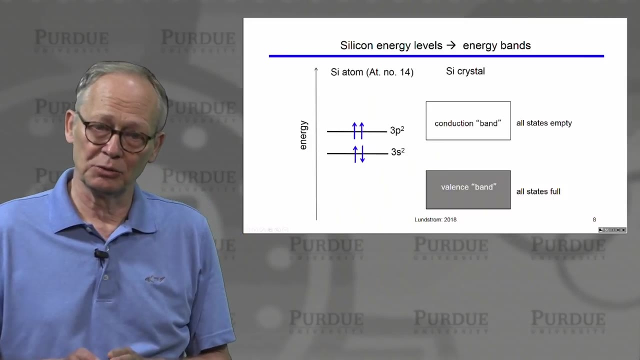 That's what holds the silicon lattice together. So there's a very important concept that happens when we put atoms together and form bonds. When we have five times 10 to the 22nd atoms per cubic centimeter in silicon, we have five times 10 to the 22nd of these states. 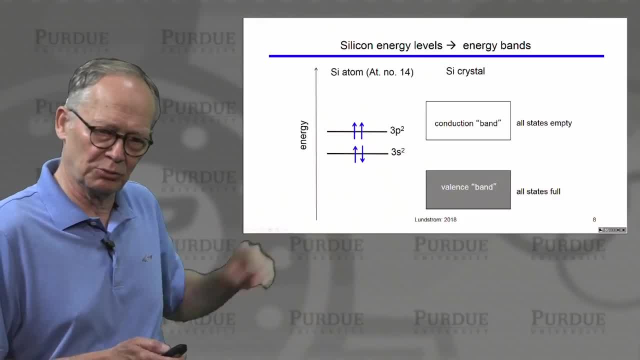 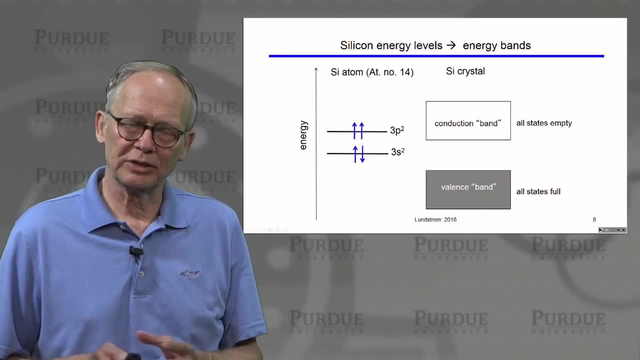 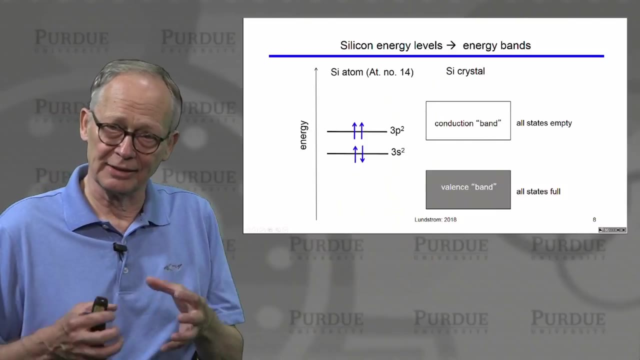 But the states change because of the interaction that occurs when the orbitals overlap and the bonding occurs. Instead of becoming discrete, they spread out and they change in energy. Half of the states lower in energy. This is what forms the energy, the bonds and that holds the silicon lattice together. 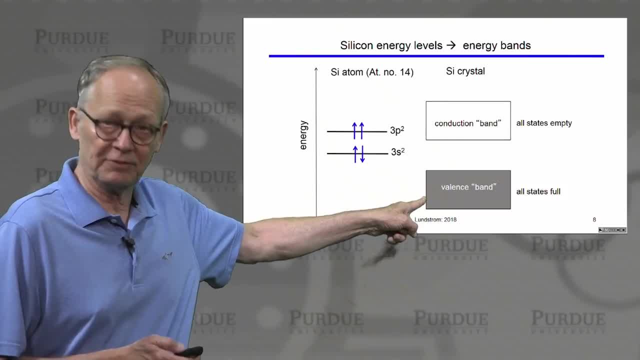 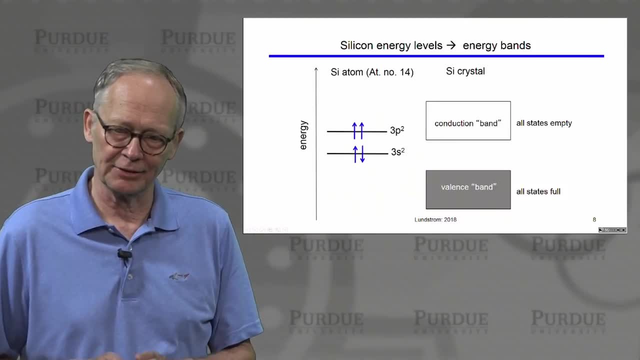 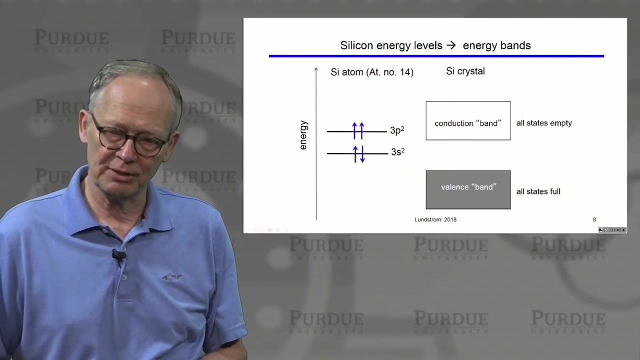 All of those states there are filled with electrons. Those are the valence electrons that are forming the covalent bonds and holding the semiconductor lattice together. Now there were also an equal number of empty states, So those empty states get pushed up in energy. 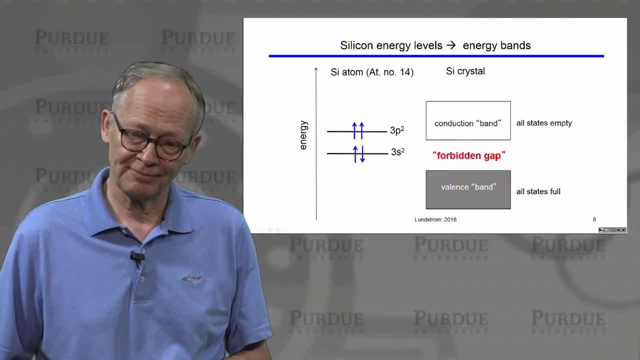 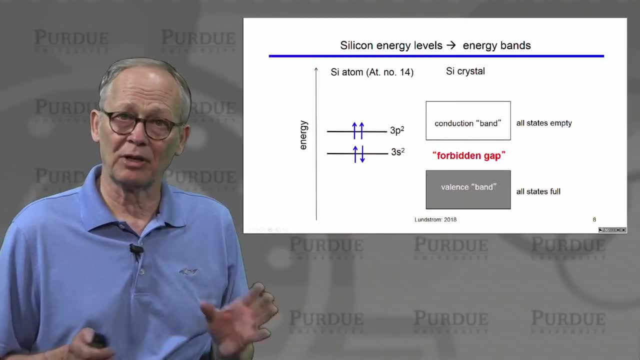 And they're available to hold electrons, but there are no electrons to hold. There's a gap between the states that are filled and the states that are empty. Inside of that gap there are no states, So no electrons can exist in that state. 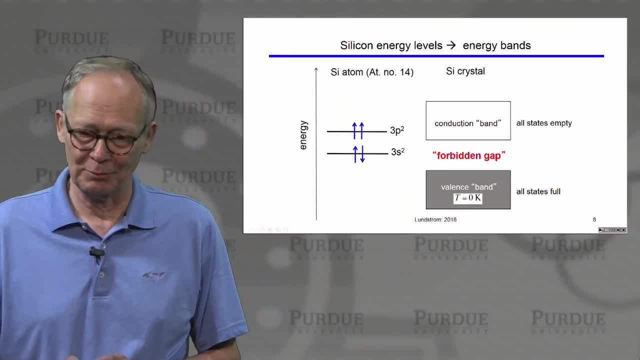 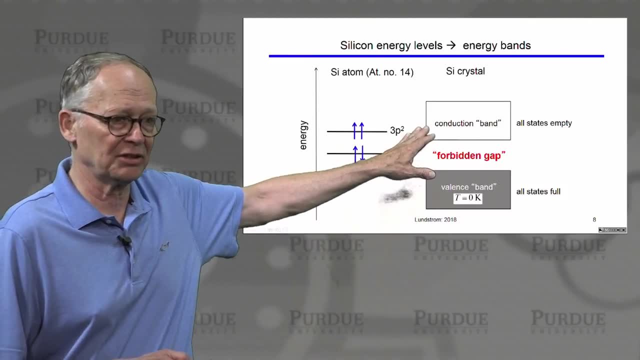 That's a very important feature of semiconductors. It's called a forbidden gap. This is the situation at zero degrees Kelvin. All of the valence band states are filled, all of the conduction band states are empty and there are no states between them. 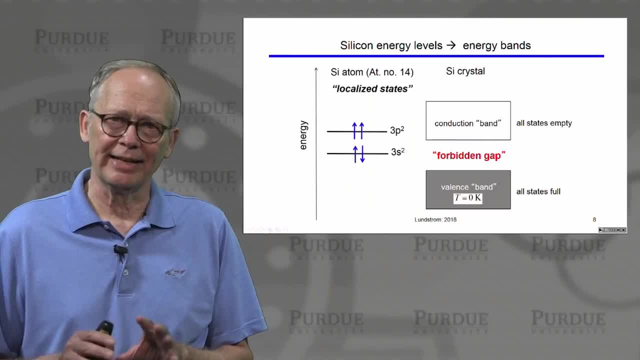 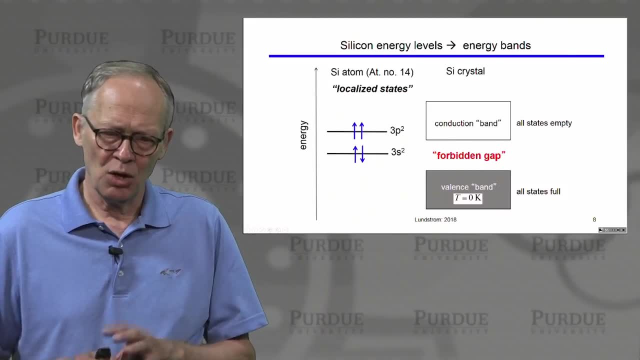 So what has happened here is that in an isolated silicon atom, the states are localized, The electrons are localized and they sit on specific silicon atoms. Once this interaction occurs in the silicon lattice between the orbitals that are very close to each other, the states become delocalized and they spread throughout the entire crystal. 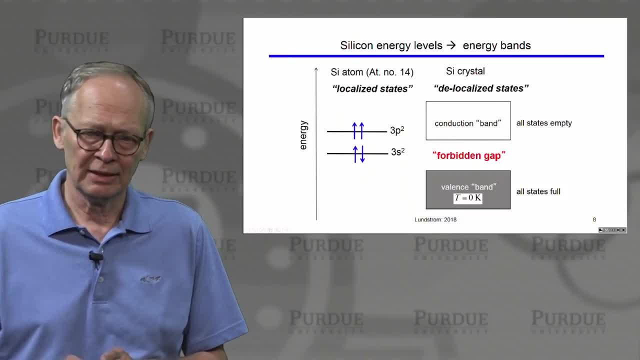 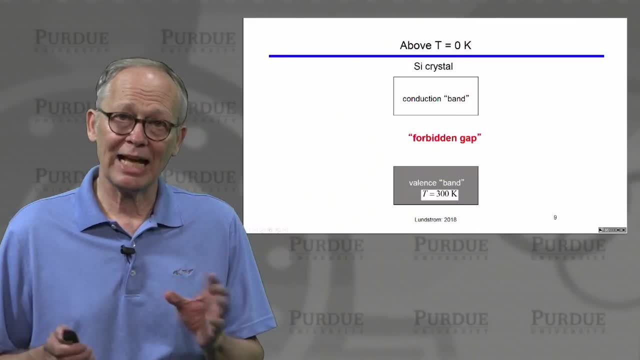 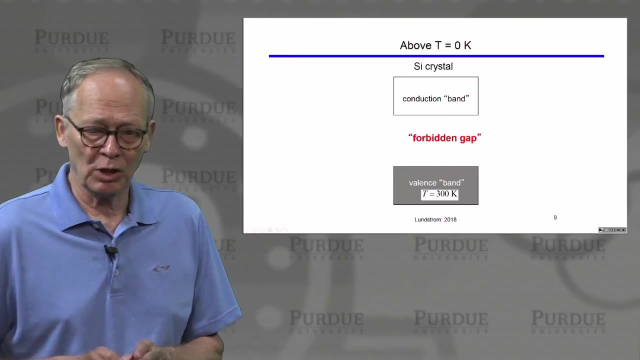 which means that electrons can move throughout the entire crystal. So that's a very important change that takes place from isolated atoms to atoms in a crystal. Now what happens if we warm the silicon lattice up just a little bit, say to 300 K room temperature? 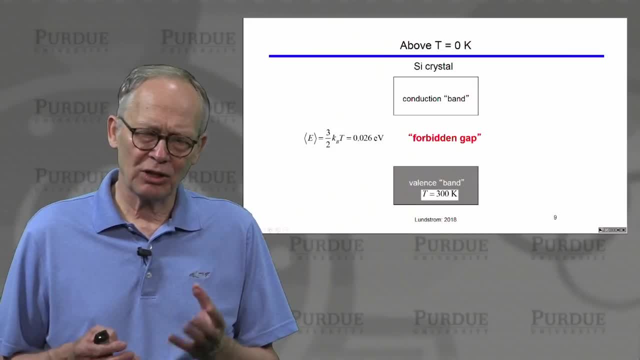 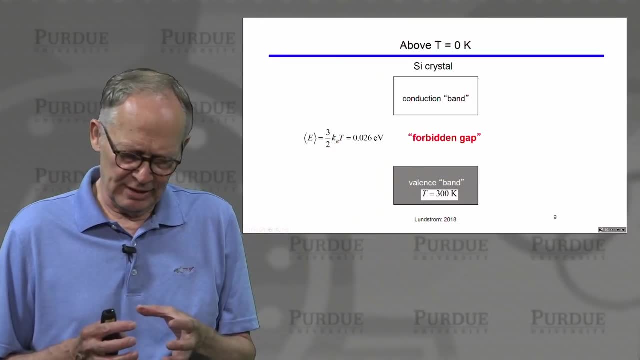 Well, if we do that, there is enough thermal energy. You may recall that the thermal energy is proportional to Boltzmann's constant times temperature. So the silicon atoms are jiggling around in random thermal motion. They have an average energy of three-halves kT. 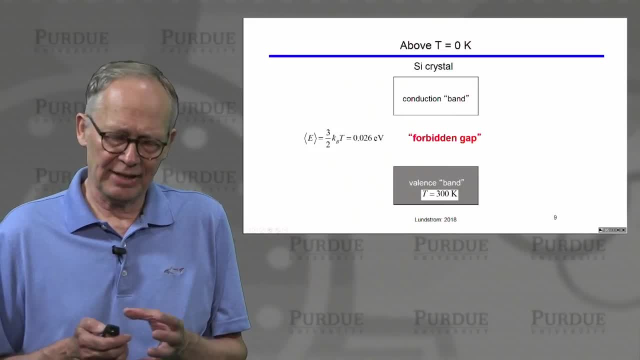 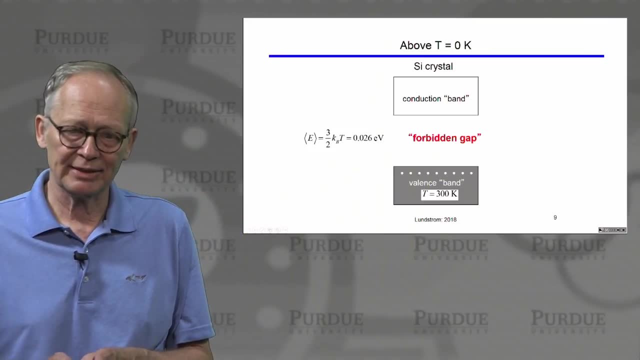 That jiggling around and that thermal energy can be enough that there is a small probability that some of those valence bonds are broken. So what happens is that when some of those valence bonds are broken, we no longer have the electron in the valence bond. 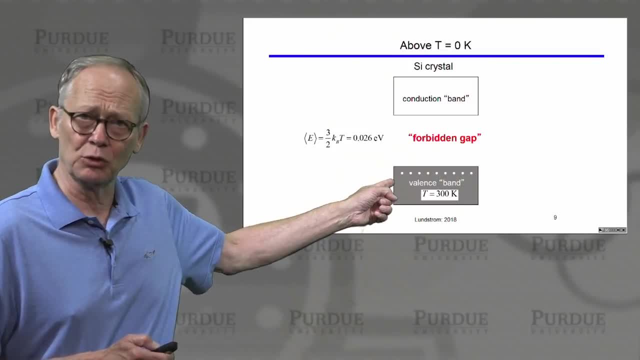 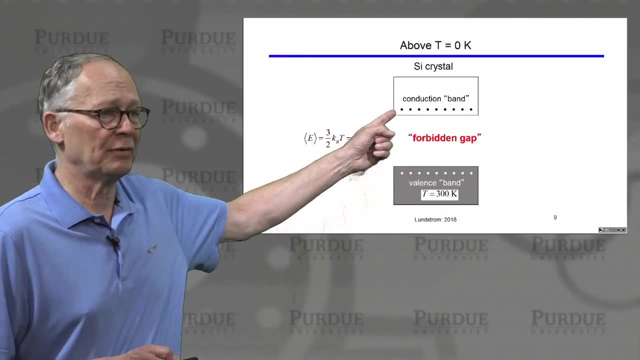 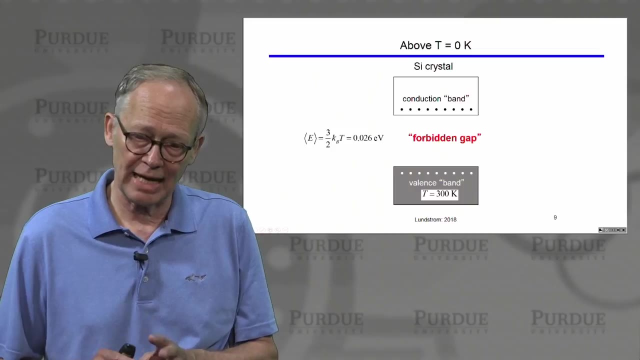 There are some empty states in the valence band, just a few. And where do those electrons go? Those electrons have gone to the conduction band. So we now have a few electrons in the conduction band. So this is the situation for a typical semiconductor crystal at room temperature. 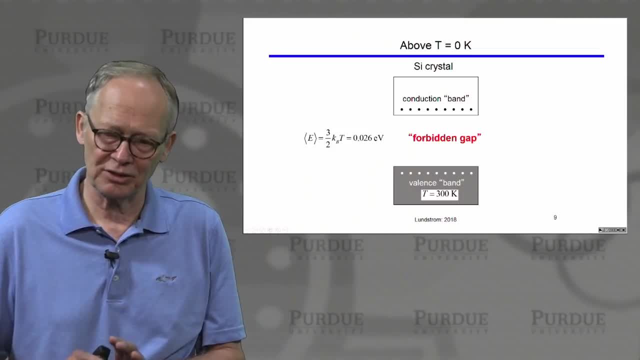 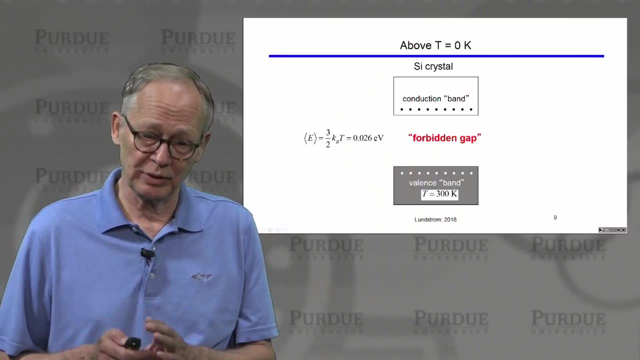 There's a large number of states in the valence band and a tiny fraction of them are empty. There's a large number of empty states in the conduction band and a tiny fraction of them are filled with electrons. So what happens? There's a large number of states in the conduction band and a tiny fraction of them are filled. 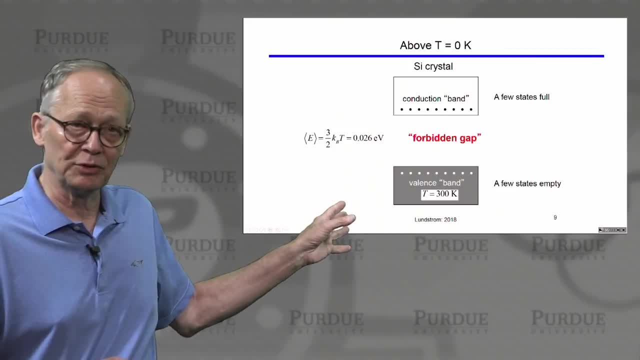 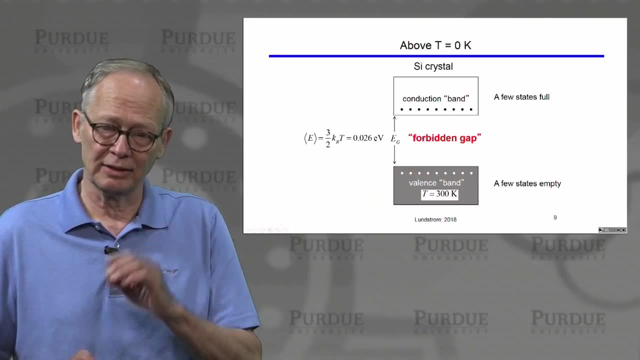 with electrons. Okay, Valence band has just a few states empty. Conduction band has just a few states full. And those two types of states, valence band and conduction band, are separated by this forbidden gap. The energy range is called the band gap. E, sub G. 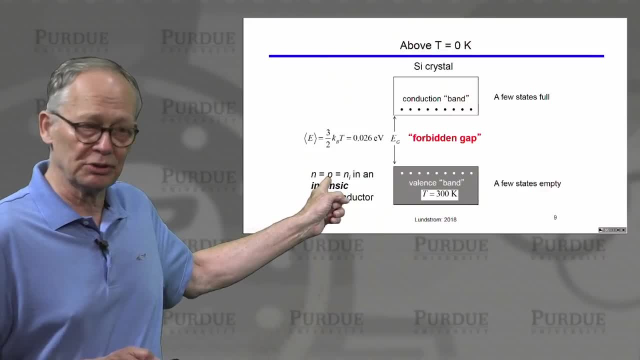 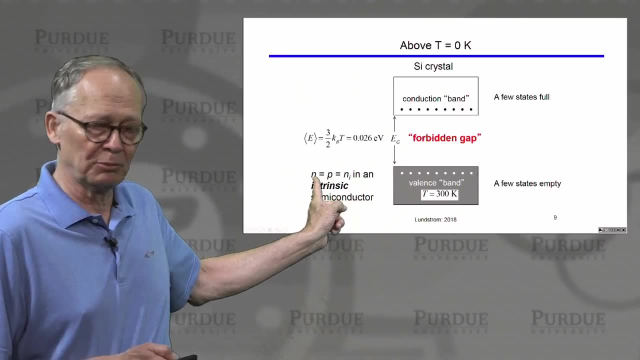 Now, since a broken bond produces a hole in the valence band and an electron in the conduction band, the number of holes in the valence band and the number of electrons in the conduction band is equal. This is a very important number. 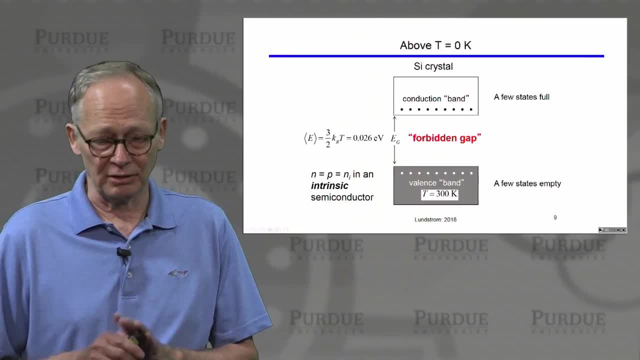 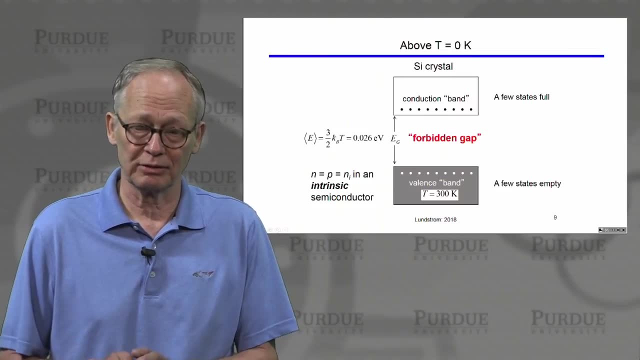 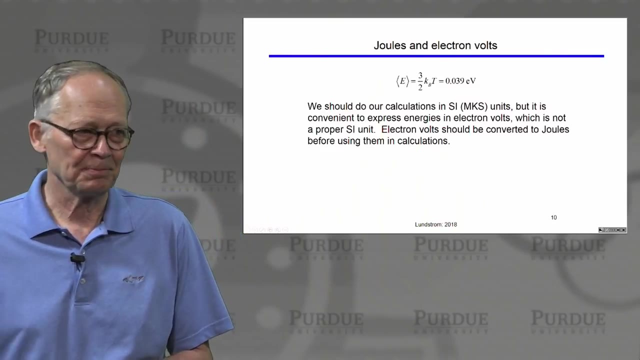 It's called the intrinsic carrier concentration. The electrons can move about in the crystal and conduct electrical currents. The holes can move around in the crystal and they can also conduct electrical currents. So the intrinsic carrier concentration, n sub i, is an important quantity. 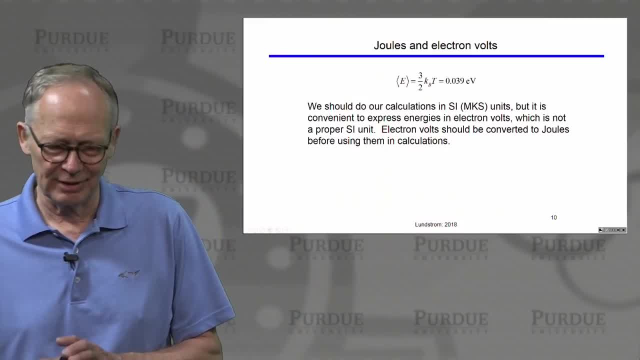 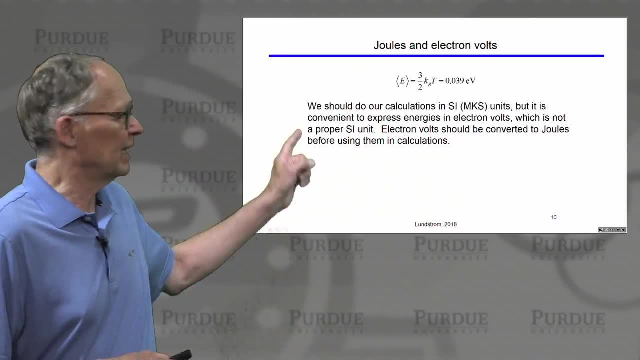 Now, as we do homework problems and work examples, there's a point that sometimes causes confusion in courses like this. So I just want to mention that When I quote energy as being three halves kT, and I quote it in electron volts, we need 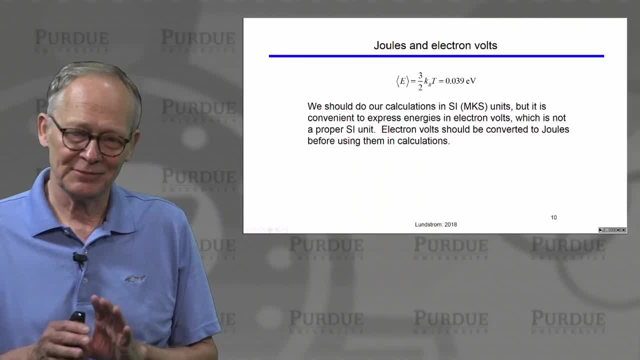 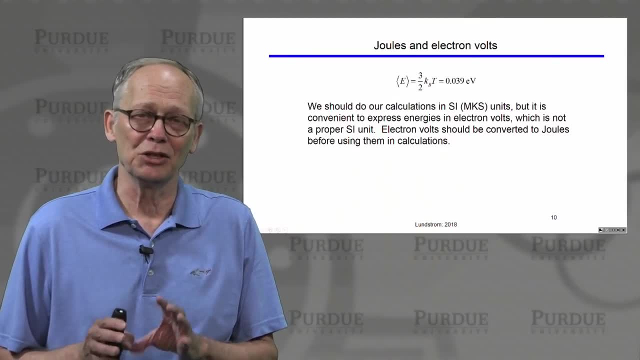 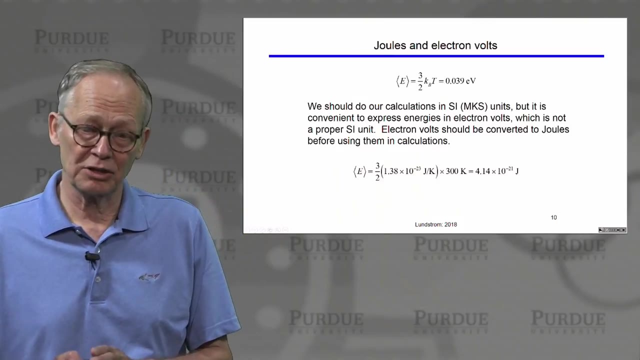 to remember that electron volt is not a legitimate unit for System, International SI or MKS units. It's a convenient unit for us to express energies in, but it's not a proper unit for doing calculations. So when we do calculations we'll have to work in a proper unit, an SI unit, and that's. 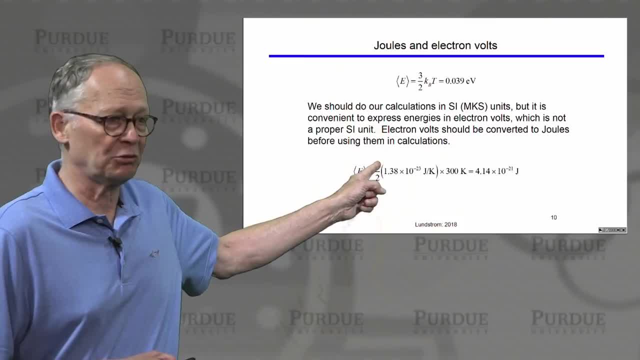 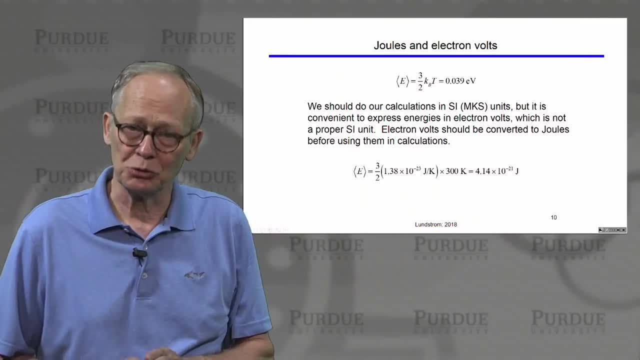 joules. So when I'm computing the average energy, I would take three halves kT. I would take three halves kT, I would multiply it by Boltzmann's constant, which is 1.38 times 10, to the minus 23rd joules. 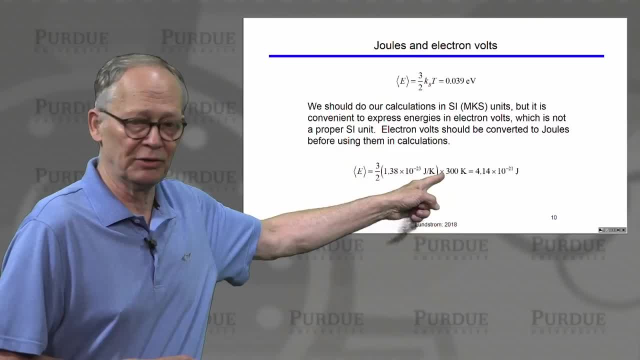 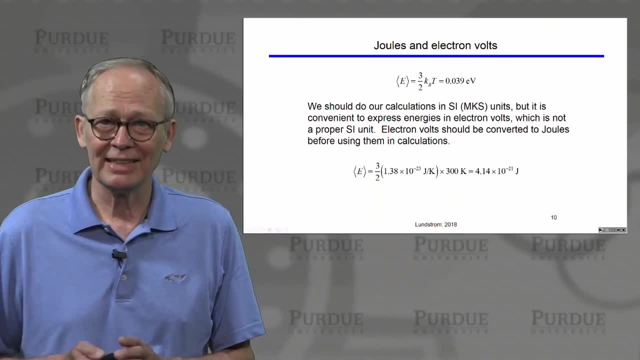 per kelvin, And then I would multiply by the temperature in kelvin 300, and the answer would come out in joules. So the average thermal energy would be 4.14 times 10 to the minus 21st joules. 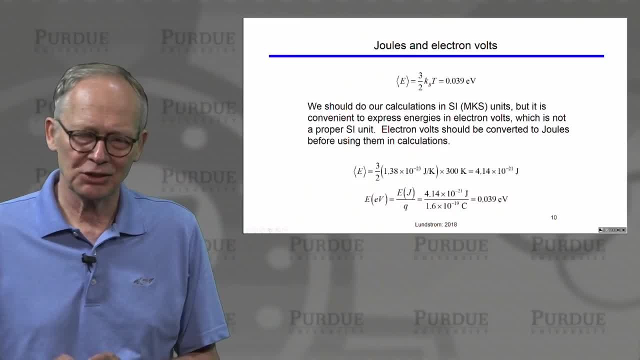 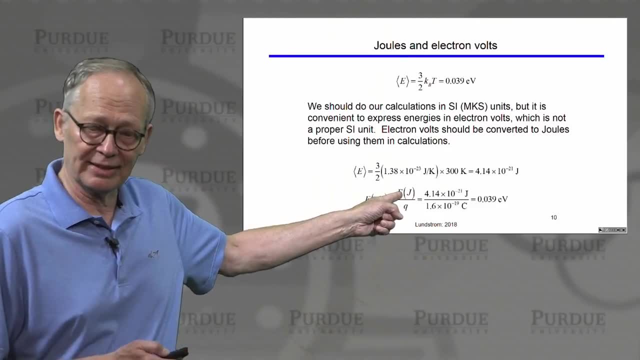 Well, that's not a convenient number to carry around in your head, So it's more convenient to think about these energies in terms of electron volts. You'll remember- It's probably physics or chemistry- that the way we convert an energy in joules to electron, 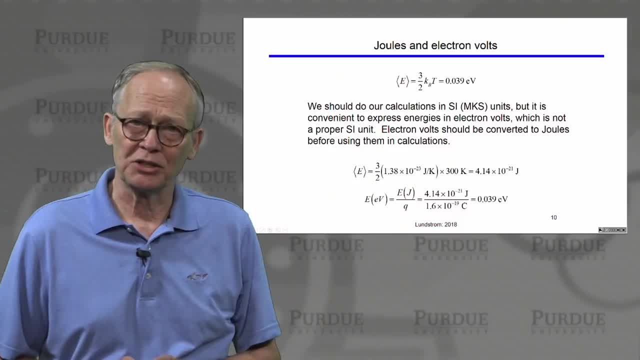 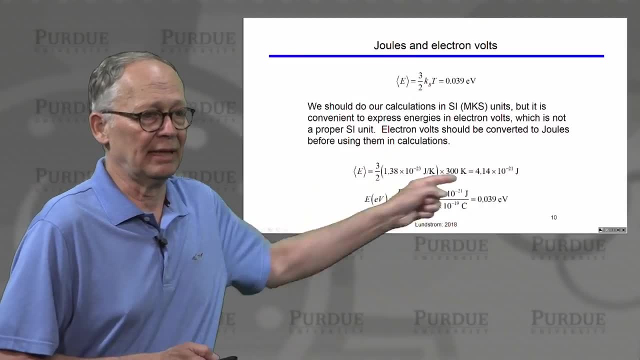 volts is: we take the energy in joules, we divide it by the charge on an electron, 1.6 times 10 to the minus 19th, and we get 0.039 electron volts. Now if I'm going to use this energy in a formula and compute something, I need to convert back. 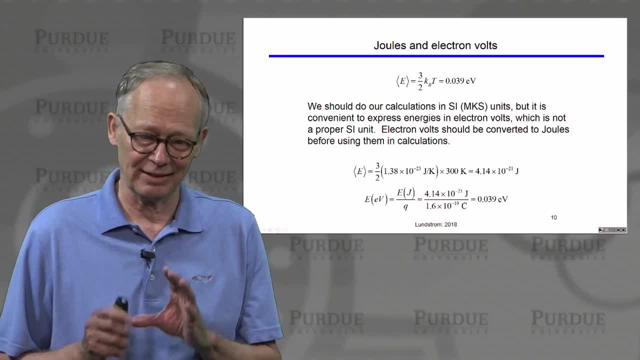 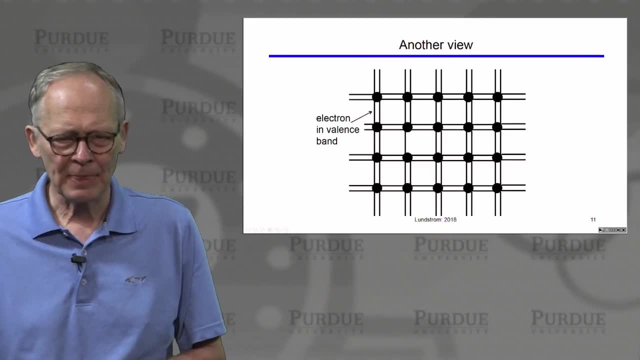 into joules and insert that into the formula. Electron volt is not a legitimate SI unit, So be careful about that. Don't do that when you're working homework problems. Okay, now there's another picture of what's happening when we break bonds and create carriers. 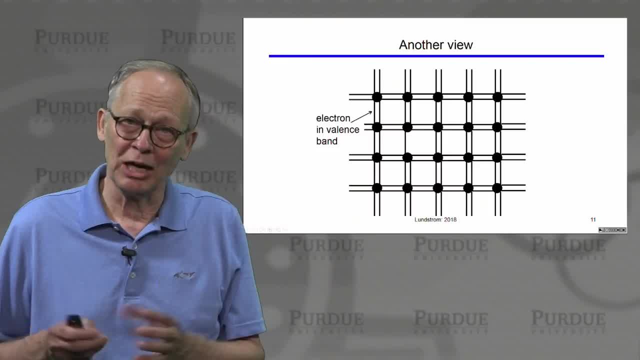 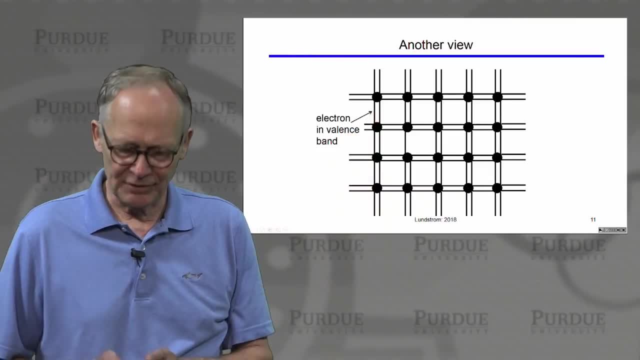 This is the cartoon of the silicon lattice. Each atom is surrounded by four nearest neighbors. The lines are the covalent bonds that hold the silicon lattice together. If there's a little bit of thermal energy, there's a small probability that some of those 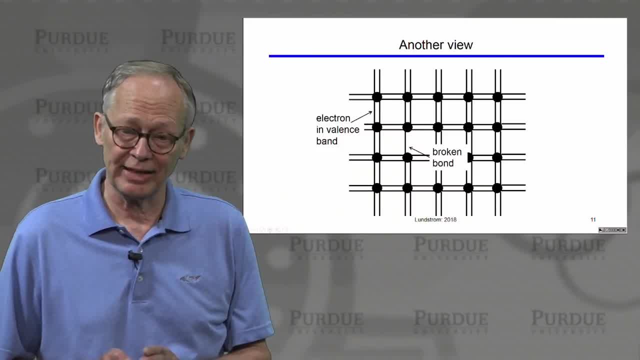 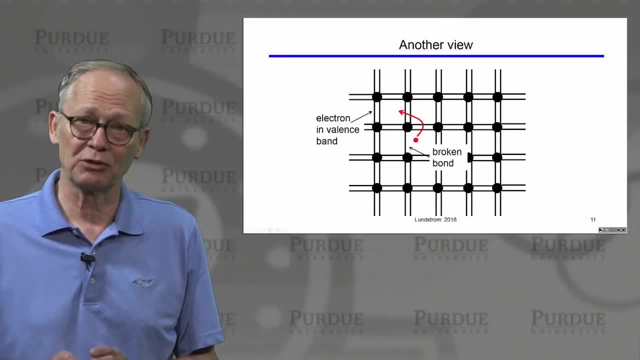 bonds will be broken. Now we've got an empty state in the valence band. What happened to that electron? That electron is now free to wander. It's free to wander around the crystal. That's an electron in the conduction band. 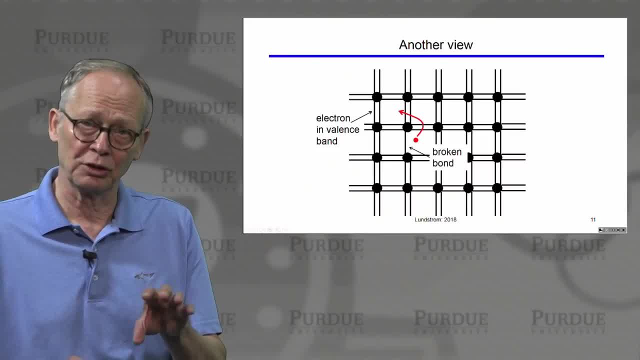 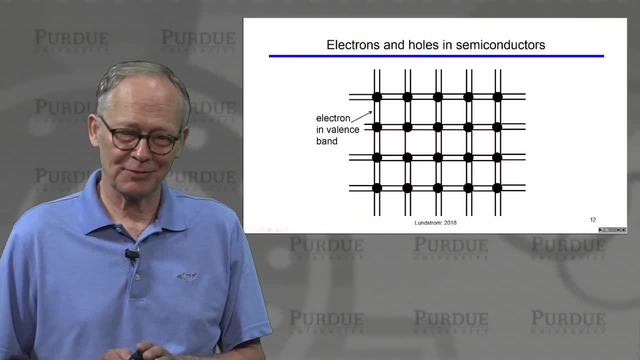 So this is an equivalent picture to the one I showed earlier with the energy band picture Now. so in semiconductors we will talk about electrons and holes. When we talk about electrons, we're not talking about the electrons in the valence band. that. 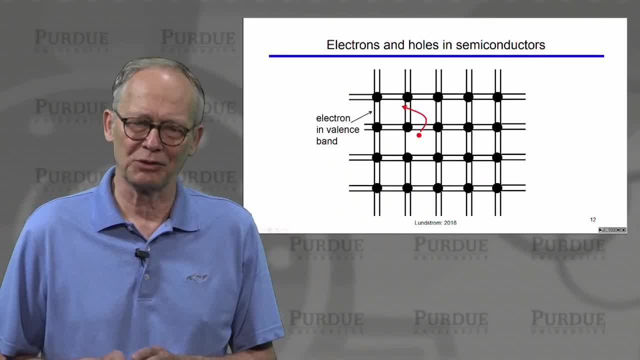 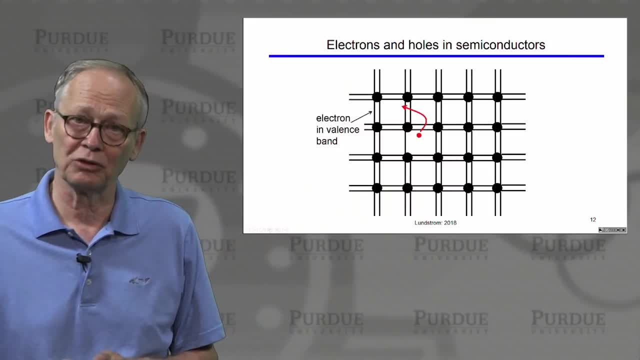 are forming the covalent bonds. We're really interested in the electrons that have been broken, that now reside in the conduction band and that are free to wander around the crystalline conduct. current We also have holes in the valence band. 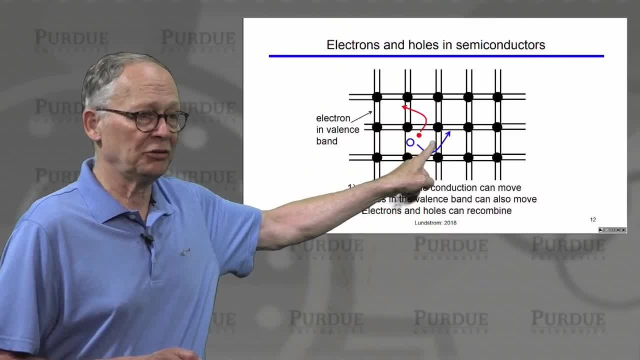 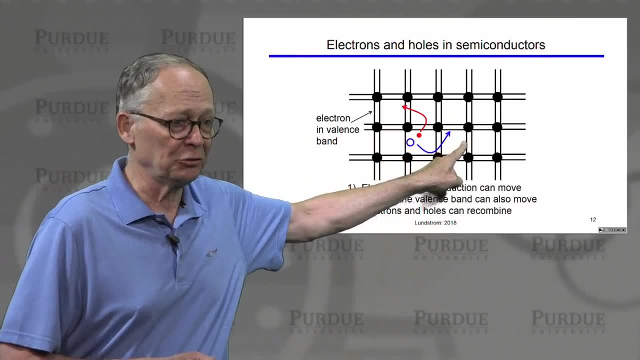 Those holes are free to move. For example, an electron in this valence band could hop over and fill up this hole. Now the hole has moved over one. Then an electron in this valence band could hop over and fill up that hole. 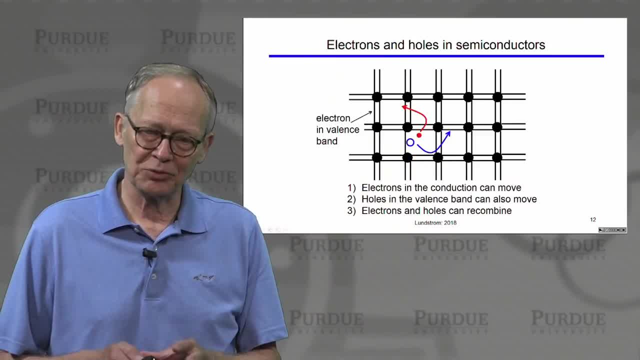 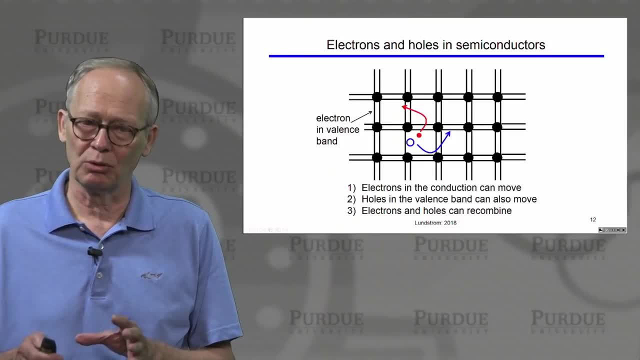 So the hole is free to move around. The hole is an absence of a negative charge, so it behaves like a positively charged particle and we will think of it as a positive charge And we will think of it as a negative charge, And we will think of both electrons and holes as being two types of charged carriers. that 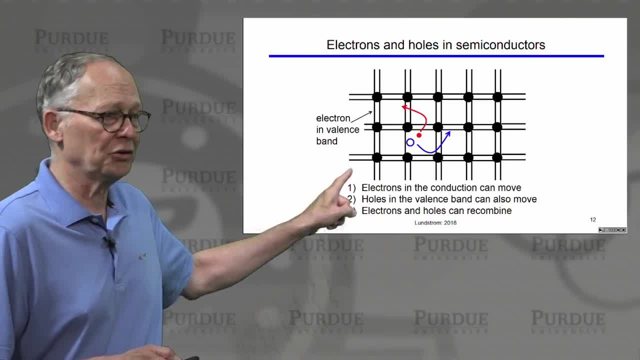 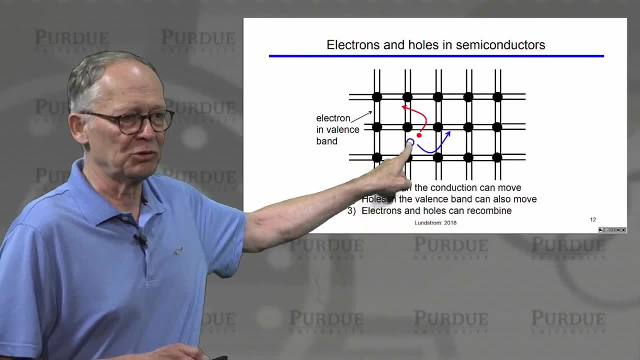 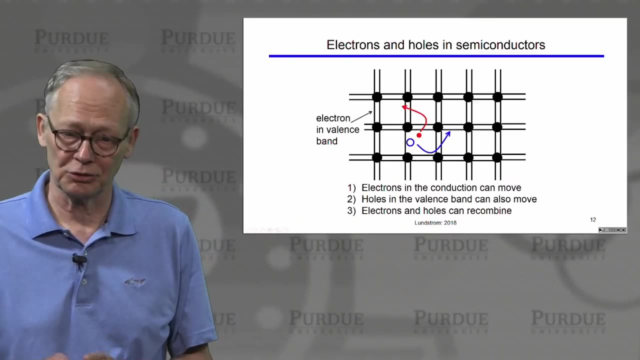 carry the currents in semiconductor devices. Now there's also another process that can happen and you can see there's nothing to prevent this electron from dropping down and filling up that hole and going back in the bond. That's called a recombination process and those occur also. 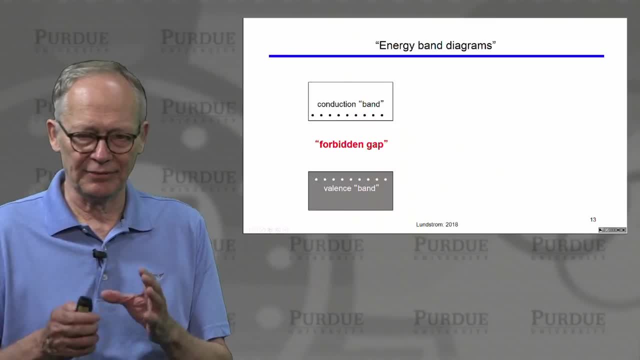 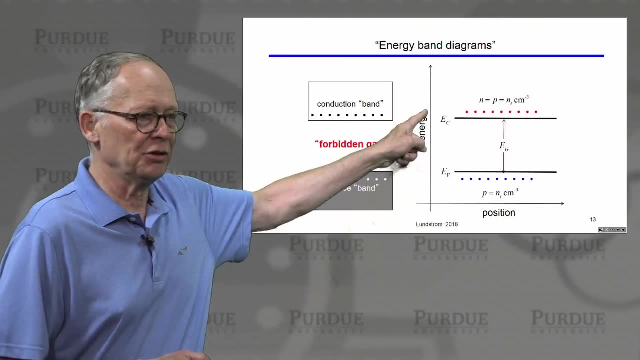 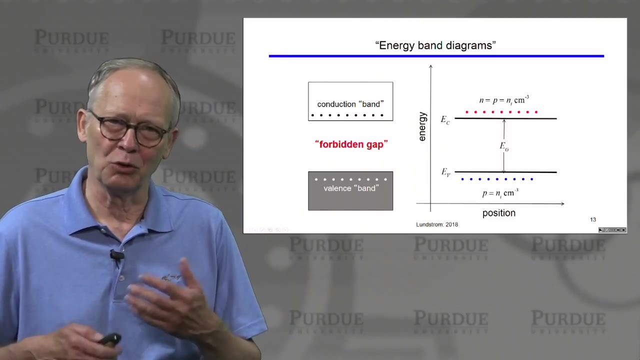 So we have this crystal lattice way of thinking about things. We have these energy band diagrams. An energy band diagram is a plot of energy versus position. But when we draw these energy band diagrams- and we're going to draw them over and over and over again in this course- we're going to simplify them. 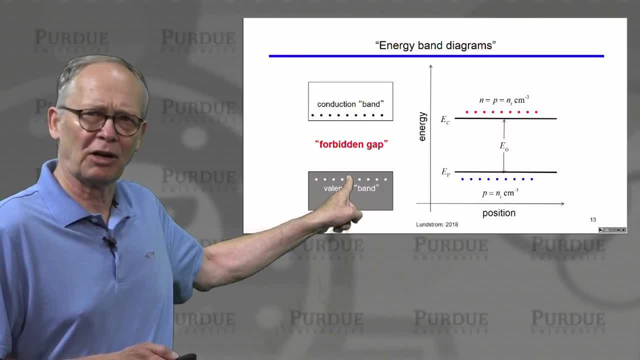 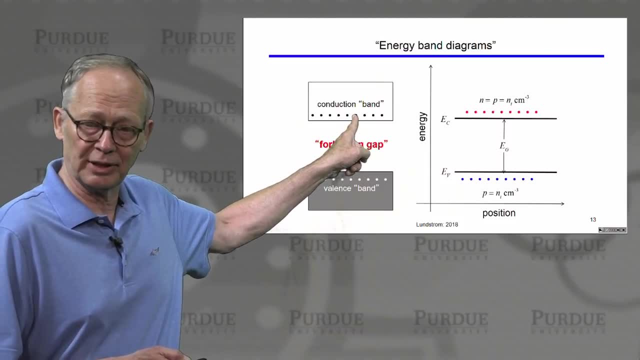 Because what we'll find is that the empty states in the valence band are all very near the top of the valence band. The filled states in the conduction band are all very near the bottom of the conduction band, So there's no point in showing the top of the valence band. 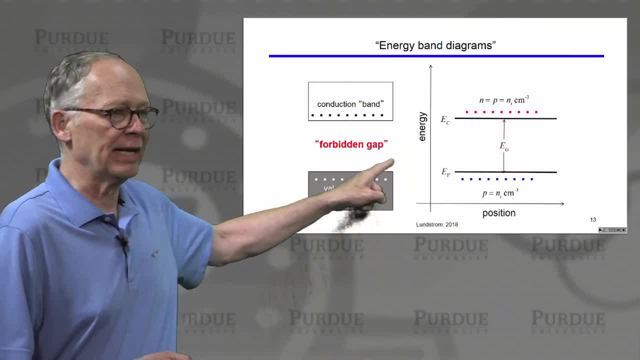 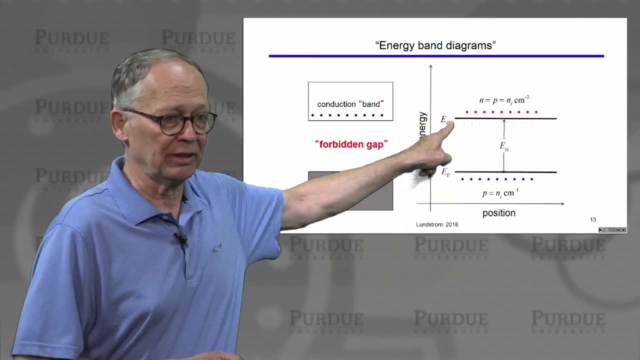 There's no point in showing the top and the bottoms of these bands. So when we draw energy band diagrams, we will simply draw the top of the valence band and we will draw the bottom of the conduction band, and they're separated by the band gap. 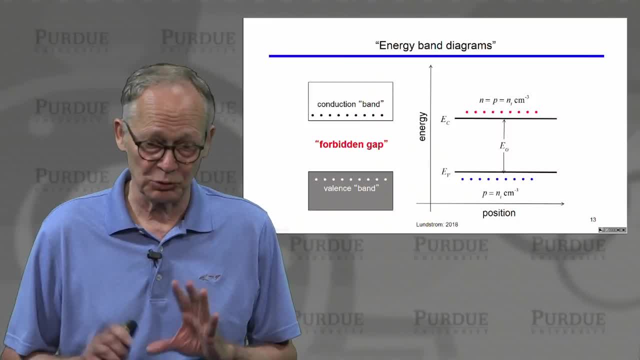 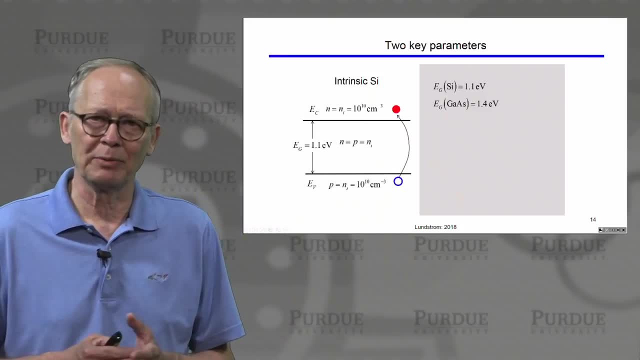 EG. That's the way we'll draw energy band diagrams, and we'll see a lot of those in this course. Now, when we're talking about semiconductors, there are many parameters that we're going to be interested in that affect the performance of a device. 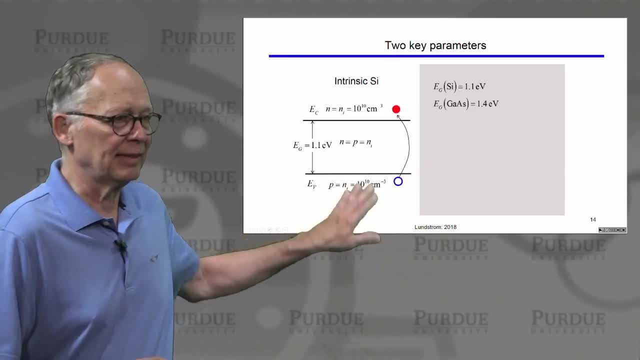 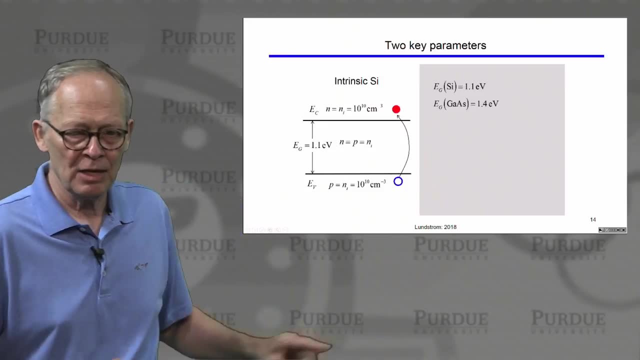 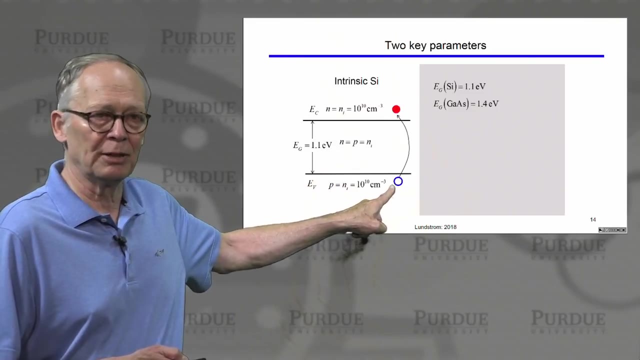 There are many parameters that we can understand already. So if this is a pure piece of silicon, we'll call it intrinsic silicon, or it might be intrinsic germanium or other semiconductors. we've seen that the thermal energy is sufficient to break a few bonds and give us a small number of holes in the valence band. 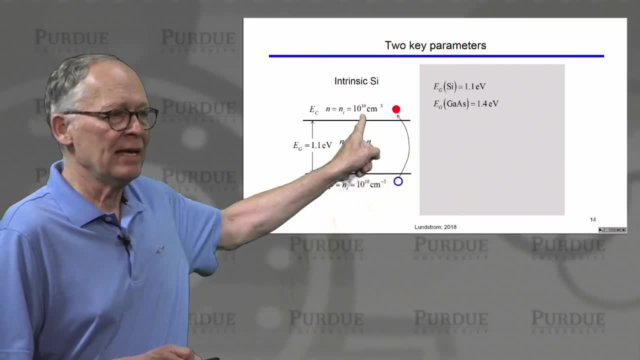 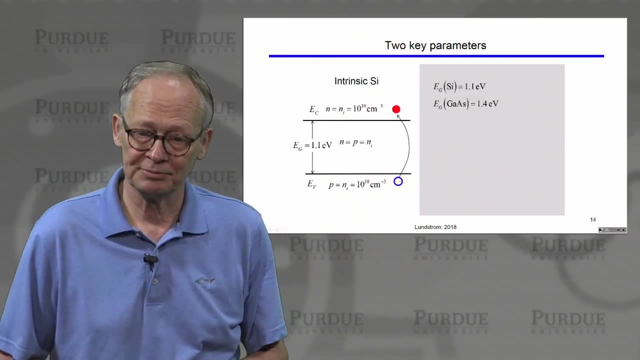 The number turns out to be about 10 to the 10th per cubic centimeter And we get an equal number of electrons in the conduction band. Same number: It's about 10 to the 10th per cubic centimeter. 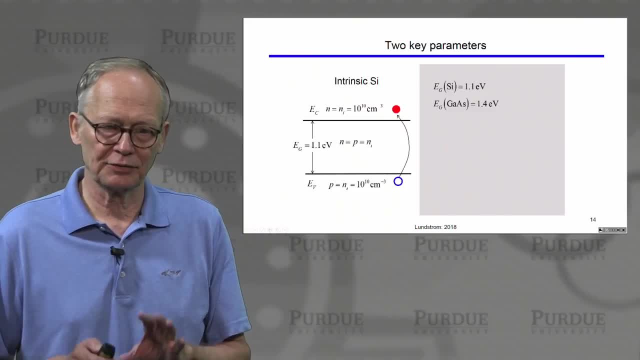 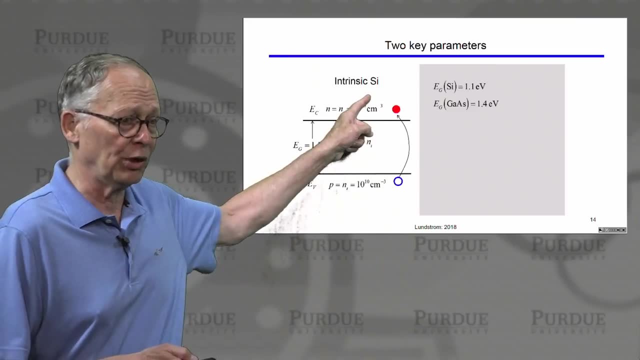 So the two parameters that are extremely important for semiconductors is: first, what is the band gap? Because that's sort of a measure of how difficult it is to break these bonds. For silicon it's 1.1 electron volts. 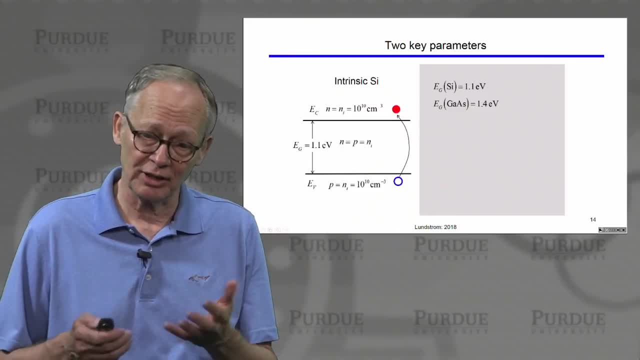 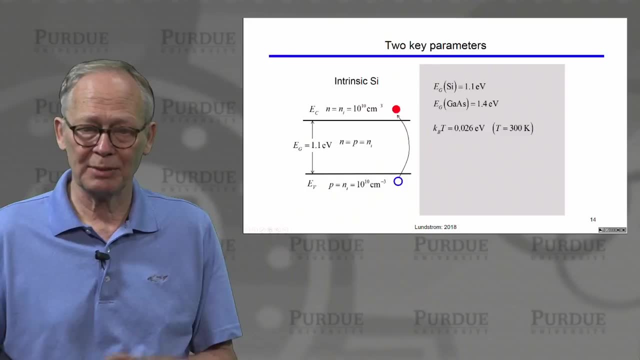 Other semiconductors have different band gaps. For example, gallium arsenide is another semiconductor. It has a band gap that's a little bit bigger. The thermal energy at room temperature, kT, is 0.026 electron volts. 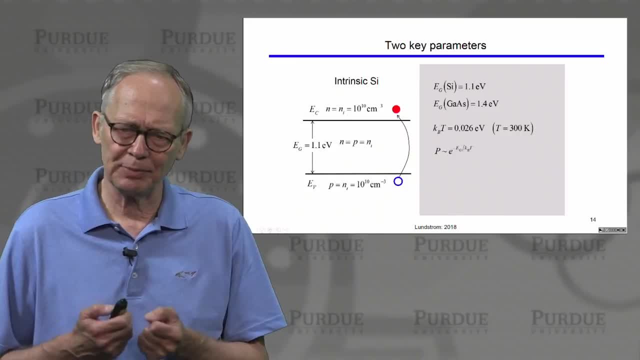 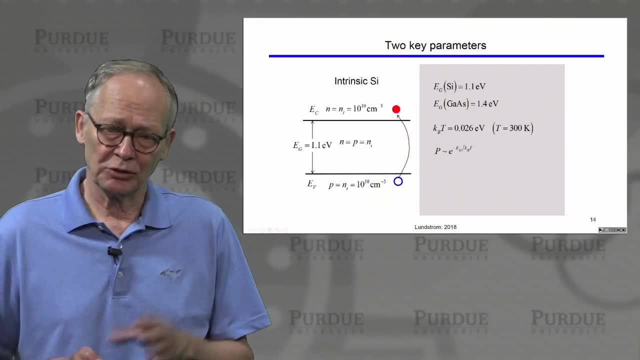 The probability of breaking one of these bonds goes exponentially with the band gap. The bigger the band gap, the harder- it is exponentially harder to break those bonds. So the number of electron hole pairs at a given temperature is extremely sensitive to the band gap. 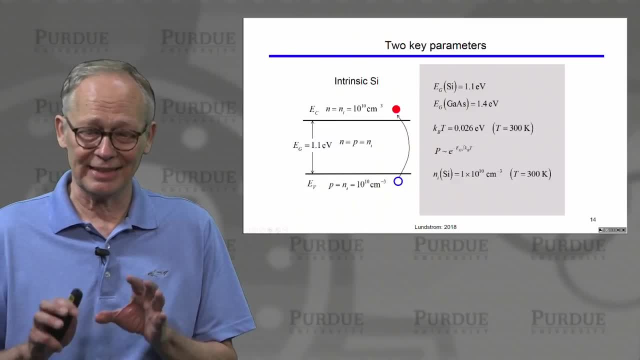 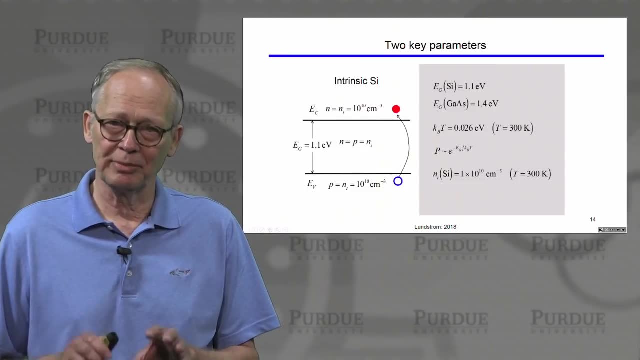 In silicon. silicon works out very nice. It's an easy-to-remember number. At room temperature, the number of broken bonds, which means the number of electrons in the conduction band. the number of holes in the valence band is almost exactly equal to the. California energy balance of these electrons. So maybe sería gustado scientifically if silicon works on these bonds. This is another example of something that can be fun to gather into the future. Okay, Let's take a look at the answer sheet. I hope everyone has a useful answer sheet. 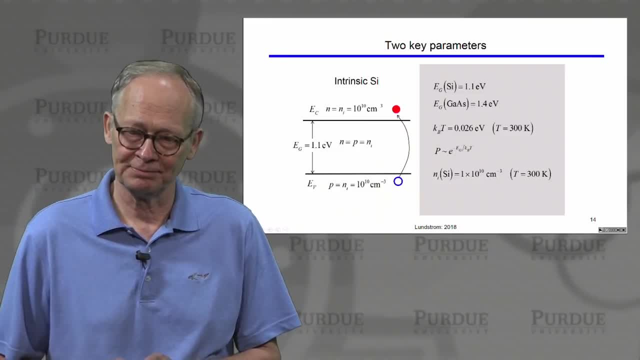 We're also happy to have a book on fees at MUAM and이라는. for each year in this, exactly equal to 1 times 10 to the 10th per cubic centimeter In gallium arsenide the band gap is bigger so it's harder to break those bonds. 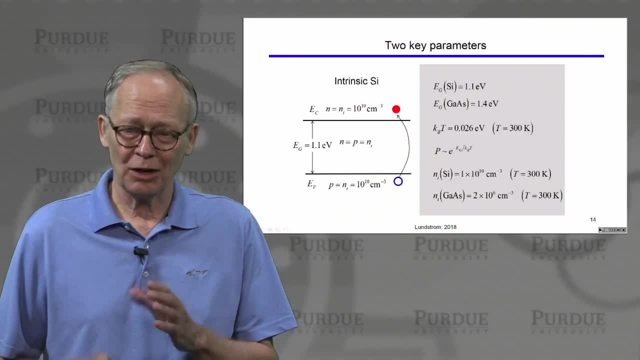 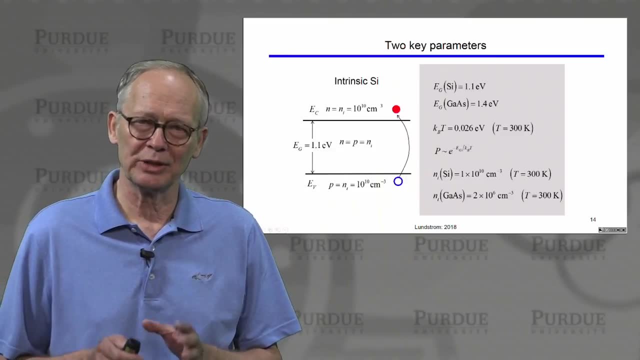 so the intrinsic carrier concentration is much less. Now, 10 to the 10th sounds like a large number, but we should be calibrated. Remember there are 5 times 10 to the 22nd atoms per cubic centimeter in a silicon crystal. 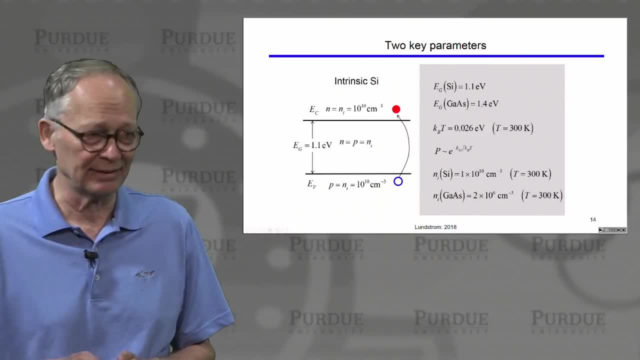 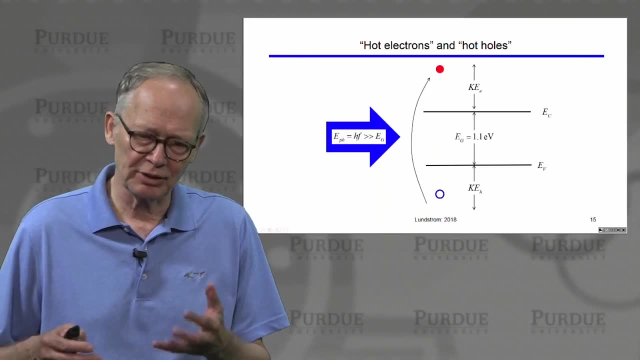 10 to the 10th is a minuscule fraction of the covalent bonds that have been broken. Okay, now there'll be some concepts that we will talk more about as the course develops, but I just want to introduce the concept here and 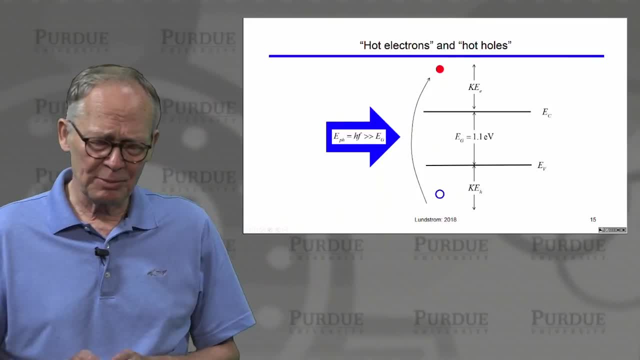 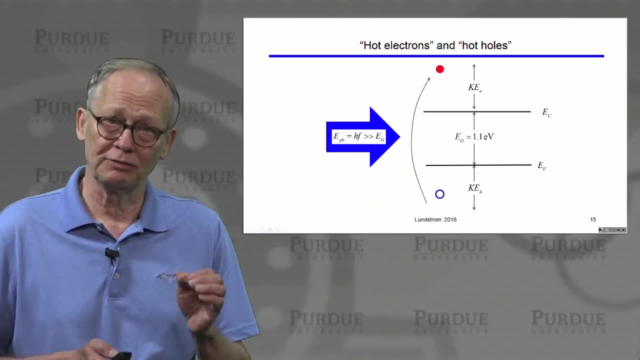 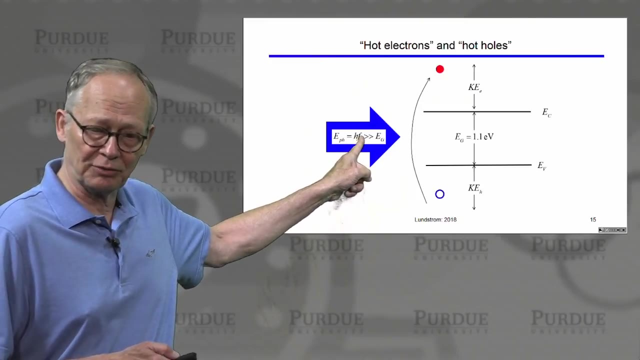 then we'll return to it later in another lecture. You'll remember from your freshman physics that light can be thought of as a wave or as a particle. The particle is called a photon. There's an energy associated with each photon. It's the energy is given by Planck's constant h times, the frequency of the light. 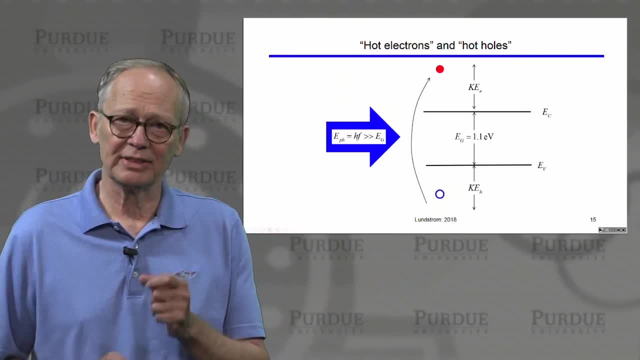 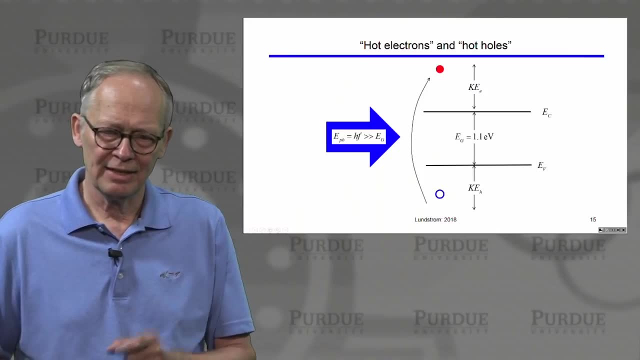 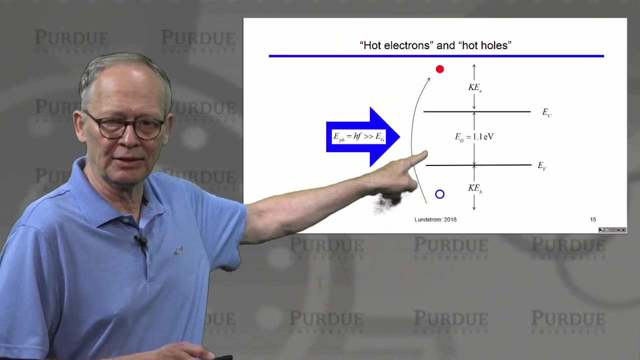 If I shine light on a semiconductor that has a frequency that's high enough, you know, or a wavelength that's short enough, so it's blue or violet or ultraviolet, then the photons will have a lot of energy And I can. I could, for example, take an electron deep in the valence band and 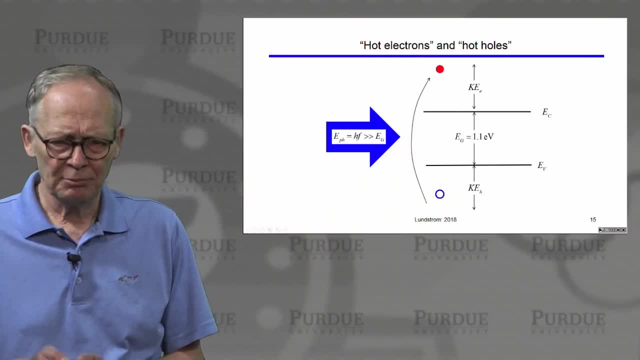 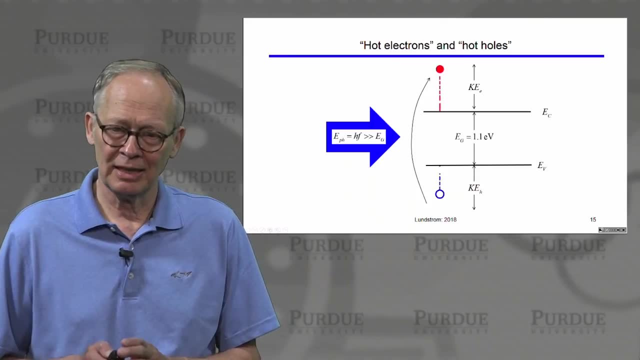 I could move it way up in the conduction band, But I said that the electrons in the holes are very near the top of the valence band or the bottom of the conduction band. so what happens? Well, what happens is very quickly. within femtoseconds, the electron will lose its energy and 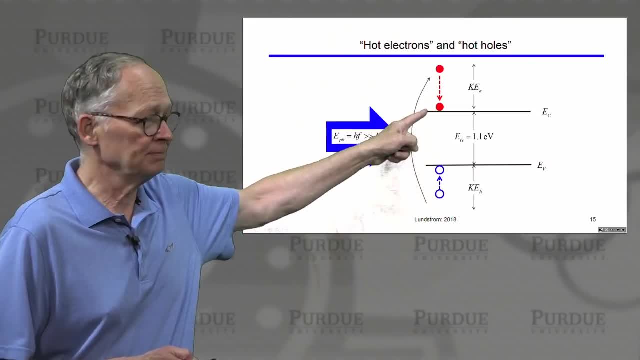 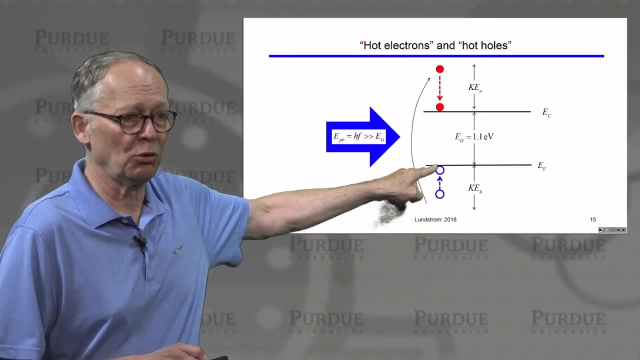 drop down to the bottom of the conduction band, then it can't drop any further. What'll happen in the valence band is that electrons in the valence band here will drop down and fill up the hole, so the hole will move up. 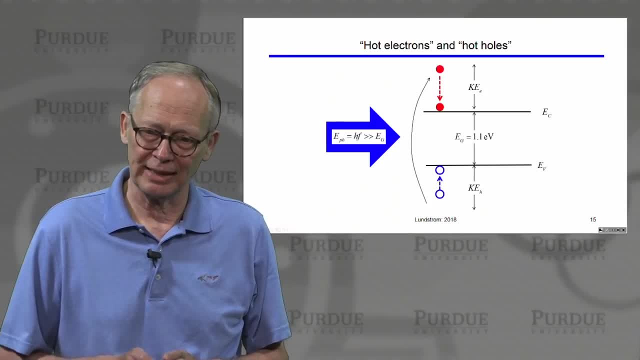 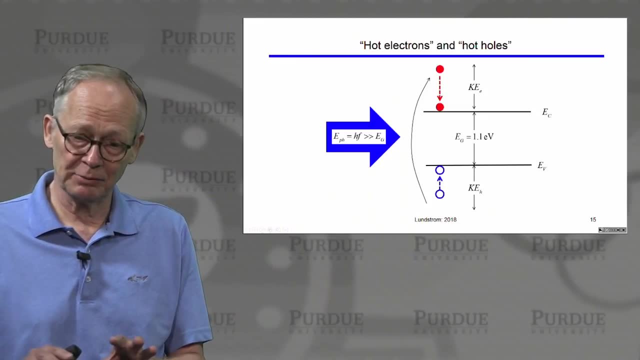 And within a few femtoseconds it will be near the top of the valence band. So we will assume in this course that the carriers are always near the bottom of the conduction band for electrons or near the top of the valence band for holes. 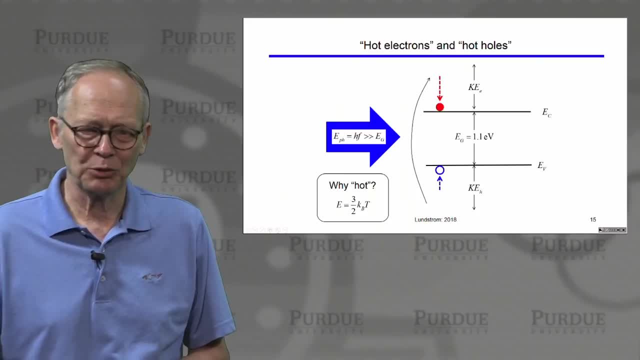 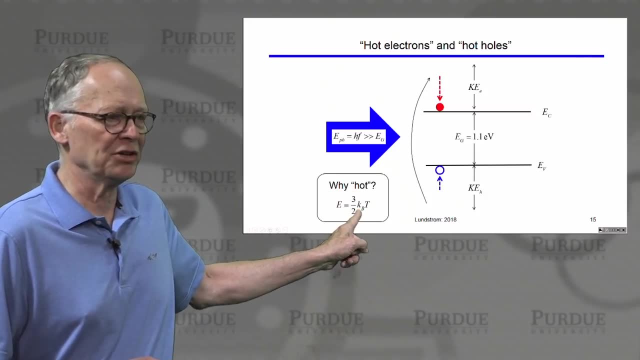 And that'll be a good assumption. By the way, the reason we would call these hot carriers before they relax to the band edges is because we like to sort of think about energy and temperature. Temperature is a way of measuring the energy of a carrier. 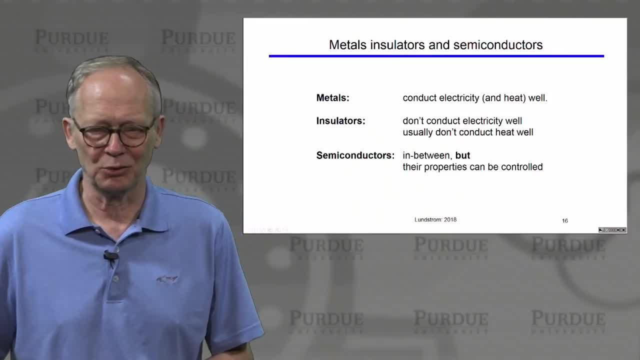 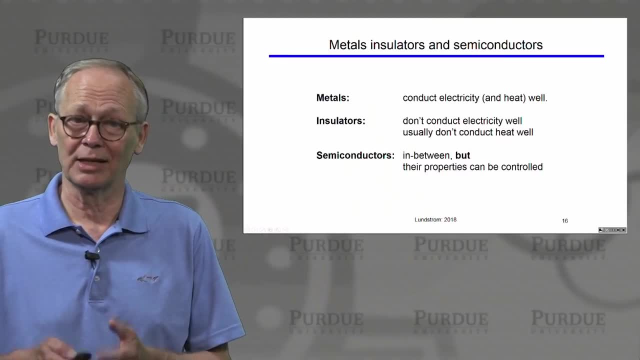 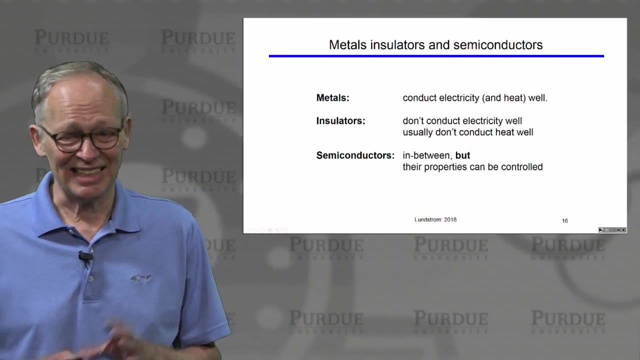 So when we're talking about effects like this, we talk about hot electrons or hot holes. Okay, we now have the background that we can understand what makes a metal, what makes an insulator and what makes a semiconductor. You'll recall, metals conduct electricity well. they usually conduct heat well also. 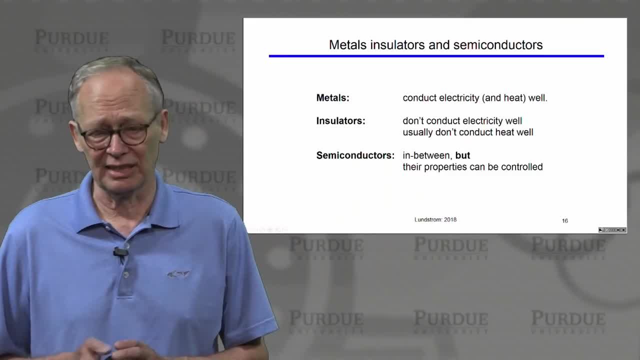 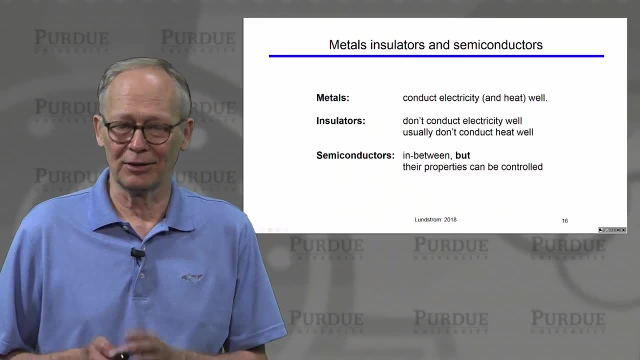 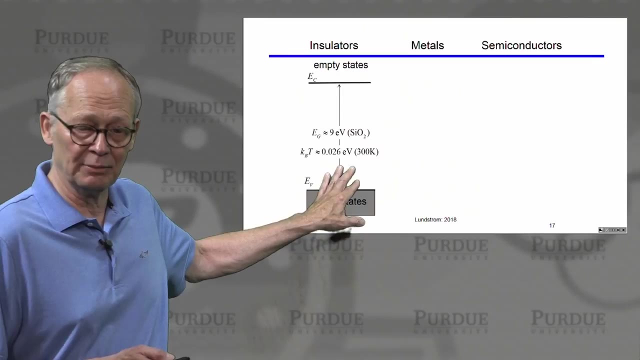 Insulators don't conduct electricity well, and they usually don't conduct heat very well either. Semiconductors are somewhere in between, but the very important property they have is that their properties can be reproducibly controlled. Now the way we would show an insulator on an energy band diagram. 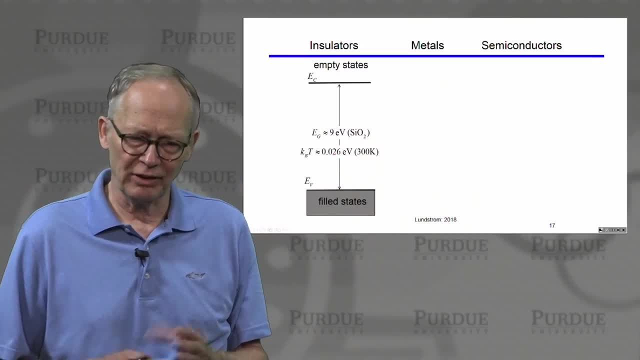 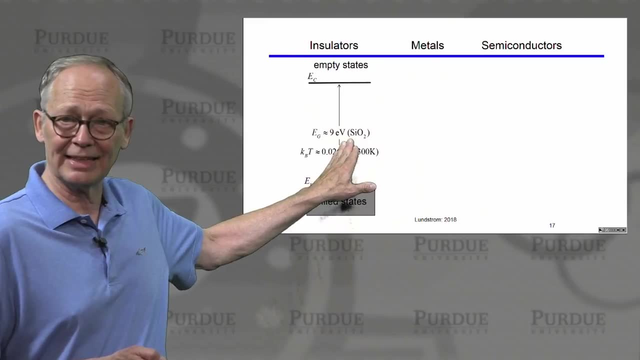 is, we'd show a material with a very large band gap. It's very difficult to break the bonds and create any carriers that can conduct current. For example, silicon dioxide, which is glass, has a band gap of about nine electron volts. Remember silicon was 1.1.. 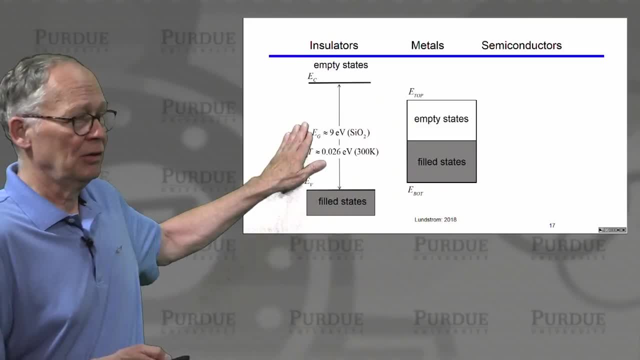 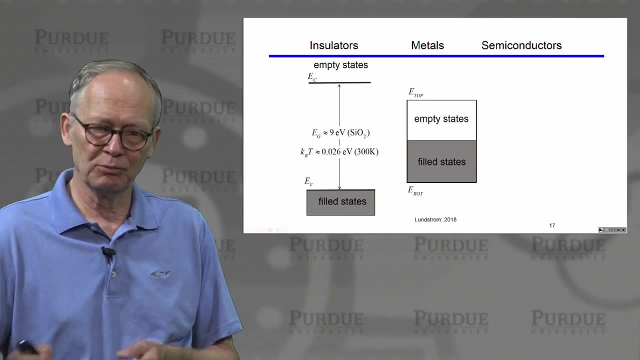 The way we show metals is: there's no band gap at all. We fill up some states and right in the middle of a band we stop and the states above it are empty. So the electrons are free to move. If they need more energy, they just move up a little bit and find another state. 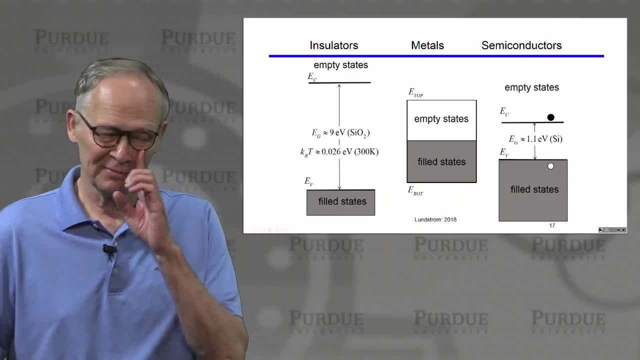 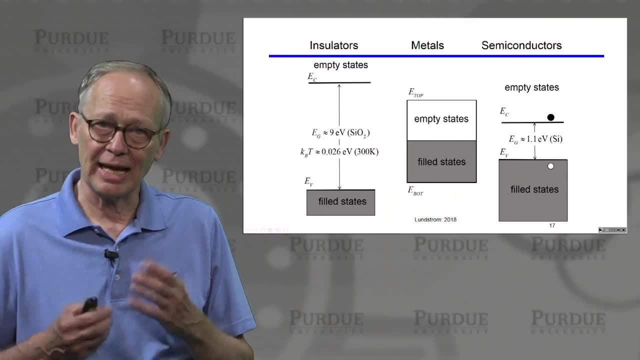 There's no forbidden gap. What's a semiconductor? Well, it works like an insulator. it just has a smaller band gap. It has a small enough band gap that, at room temperature or at reasonable temperatures, a few of the bonds are broken and 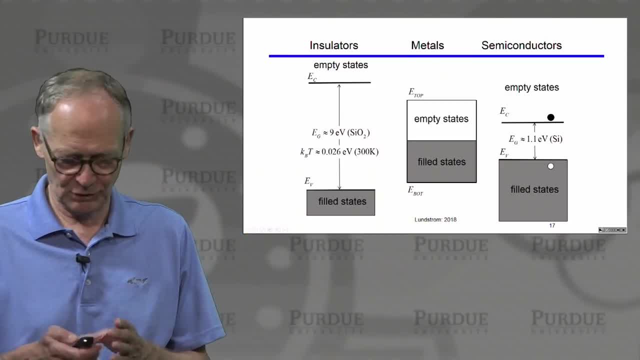 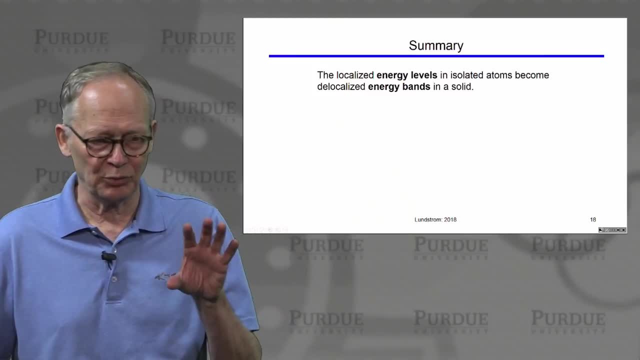 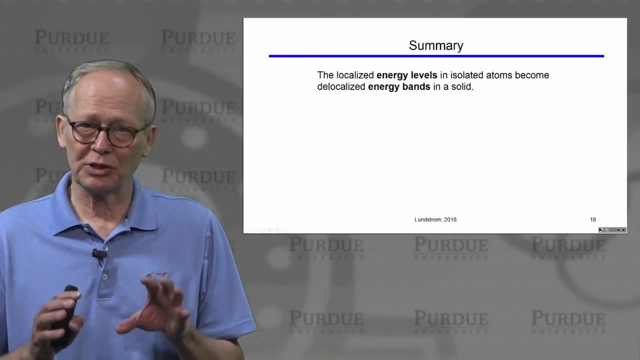 there are a few electrons and a few holes that can carry current. Okay, we have covered a lot of ground. Let's wrap up. The important concepts are that if we take isolated silicon atoms, we have a set of discrete energy levels. When we create crystals of semiconductors,